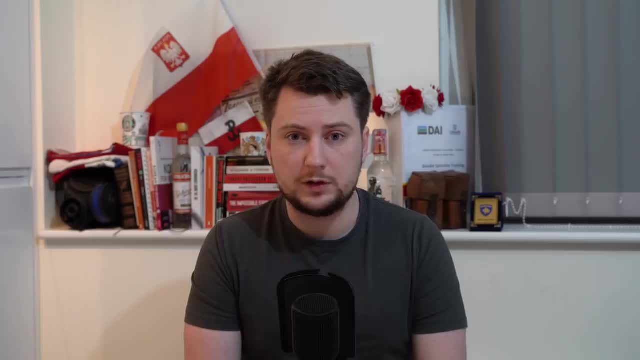 Nationalism is something that seems to really divide East and Western Europe. In the West, patriotic feeling and national sentiment seem to have become something taboo, especially after World War II, And in Eastern Europe, especially in Poland, it seems to be something that's. 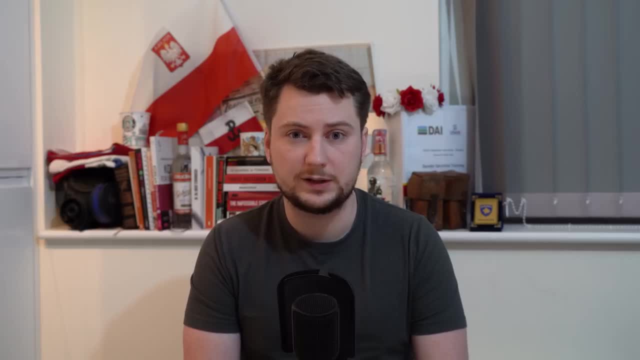 celebrated Most starkly. this can be seen in the Polish Independence Day march, which has become a holy land meeting point for writers all over the European world who want to marvel at it. So I thought I'd go there and see what all the fuss is about. 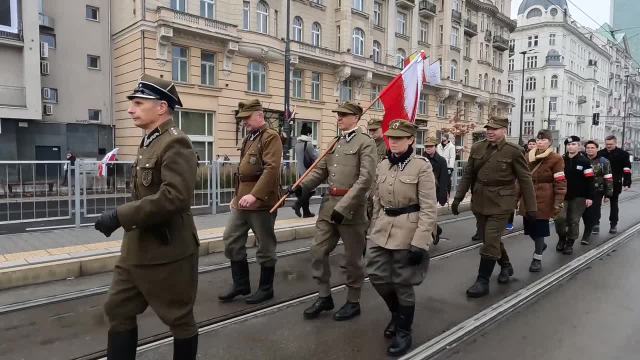 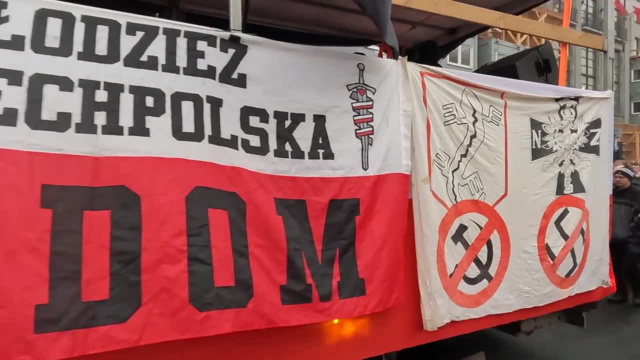 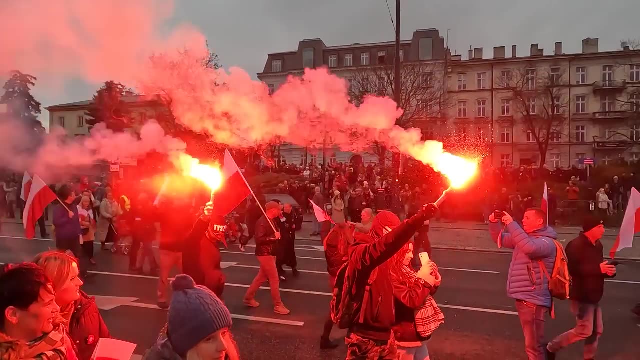 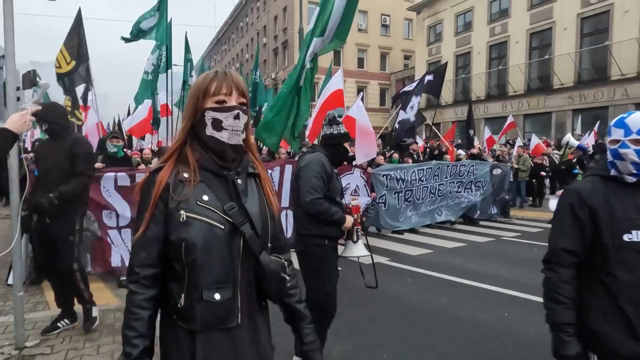 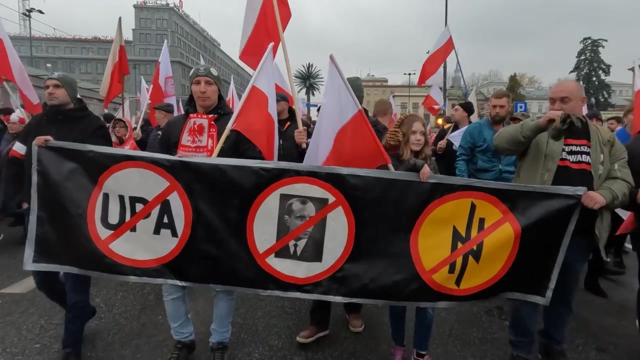 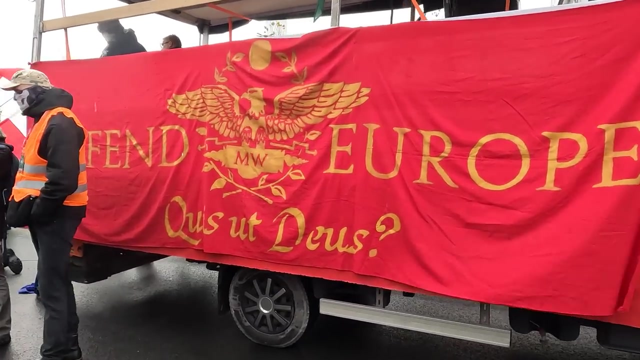 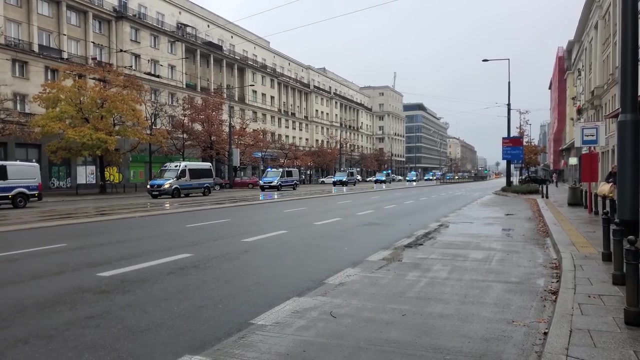 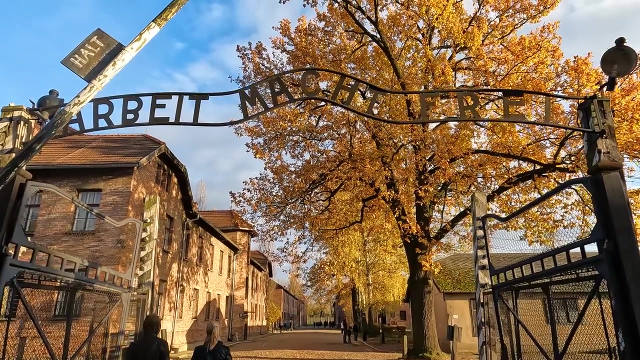 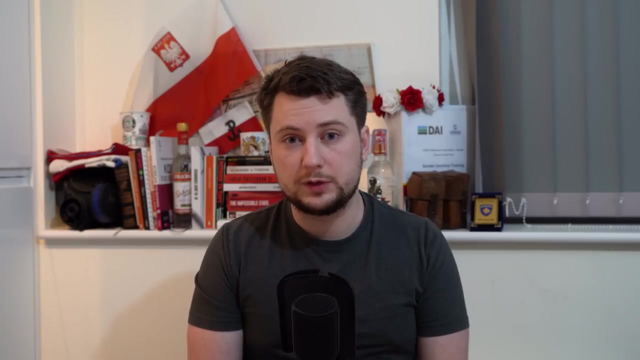 Thank you. Thank you. Normally when I visit a country, I like to spend as much time as possible to get to the true feeling of the place. This time I only had five days, but I was able to visit two dark tourist hotspots: the Polish Independence Day march and Auschwitz death camp. Weird trip. 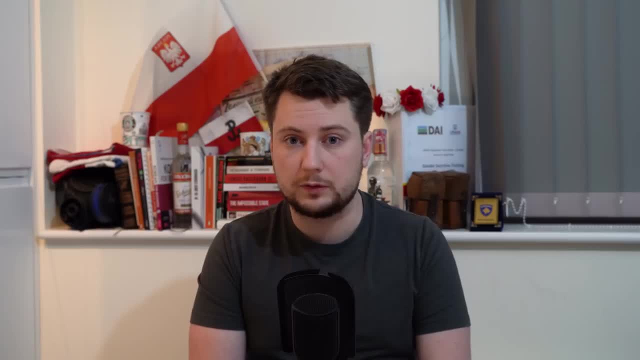 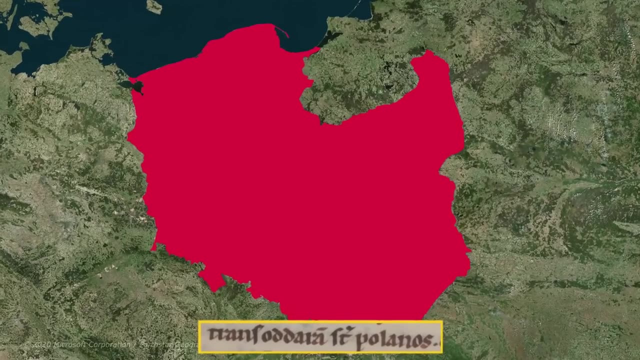 I'll admit, but I think these two places do sort of sum up the Polish experience, which has certainly had its ups and downs. References to the Polands as a Slavic tribe go back to the 700s, and the first Polish state, the Duchy of Poland, was founded in 966.. 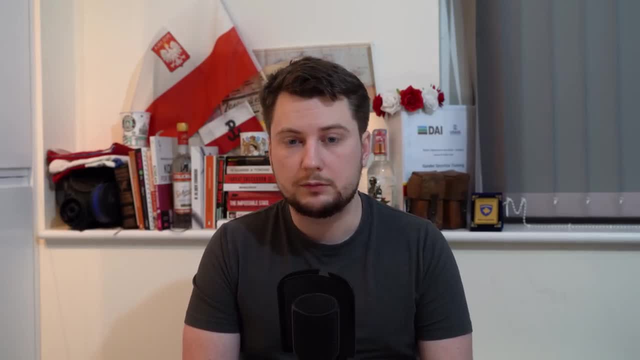 If we went over everything, we'd be here for well over an hour, but the short version is that they are one of the many indigenous ancient ethnic groups of Europe. So here's the cliff-notes version. After founding the Kingdom of Poland, this ended up becoming the massive Polish-Lithuanian. 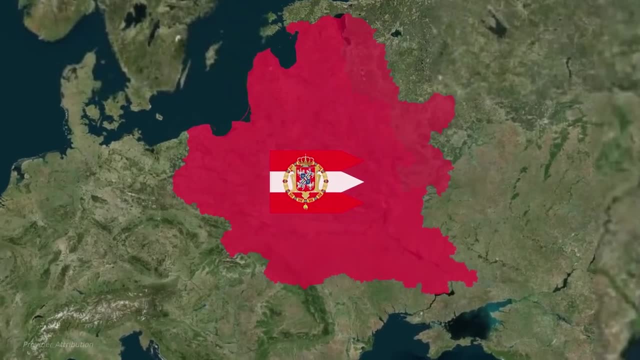 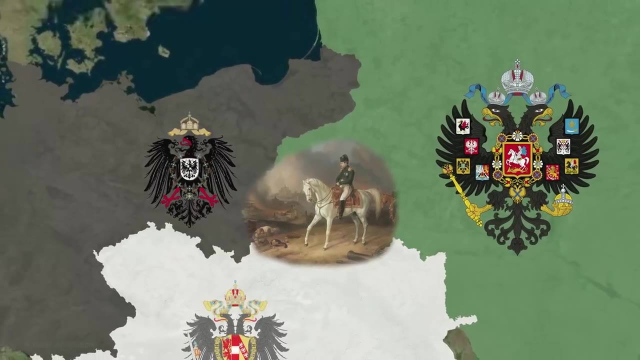 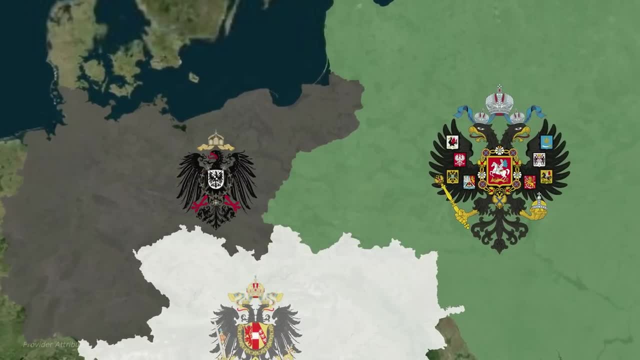 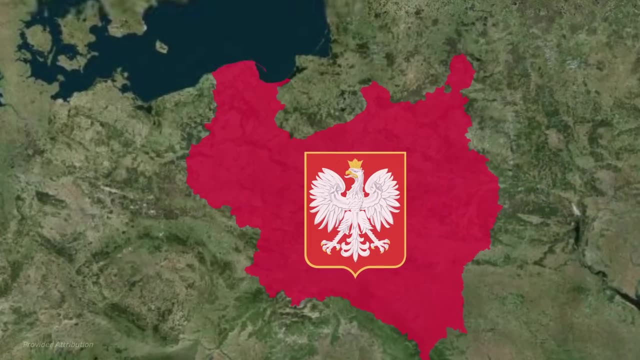 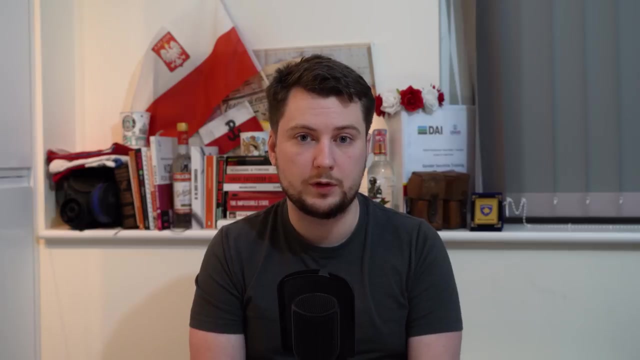 National Anthem. During WWI there were Poles on both sides, as Russia and Germany both collapsed and Polish nationalists were able to establish an independent Polish state. So on the 11th hour of the 11th day of the 11th month in the Anglosphere, we remember all those who died in great sorrow. 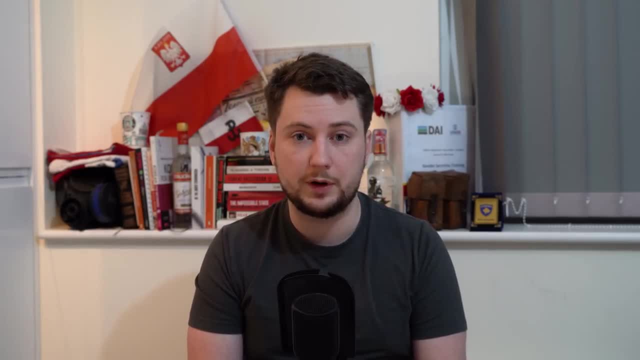 However, in Poland it is something in which there is a celebration of the sacrifice that was faced to give Poland its independence back. But now that Poland has found her independence, it would all be smooth sailing from here. No, What followed was probably the darkest period in all of Polish history. 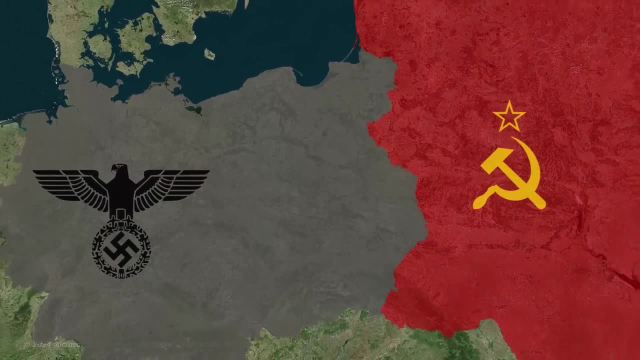 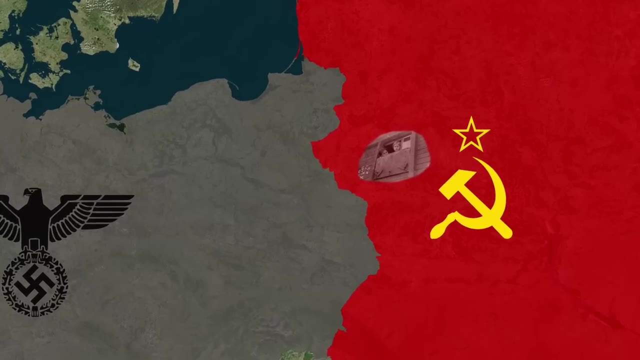 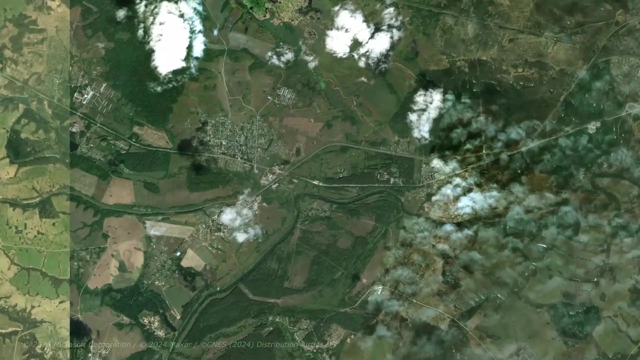 First the Germans invaded and then the Soviets joined them. The country was split in two between the National Socialists and the Communists. The Soviets deported Poles in cattle cars to become slave labour in the frozen east and rounded up 10,000 educated Poles most likely to form resistance. 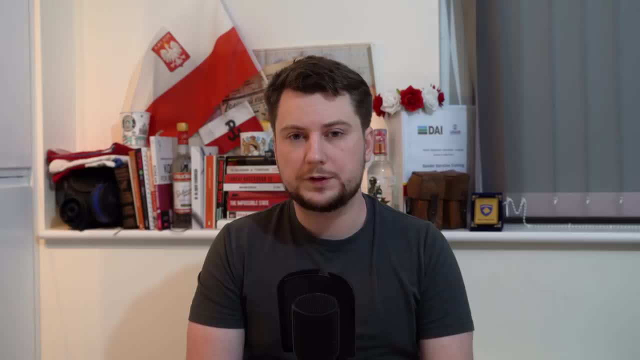 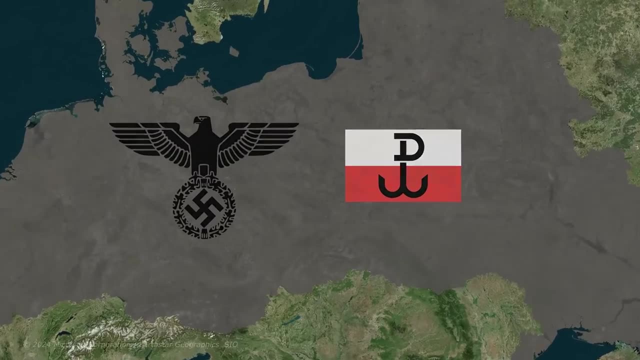 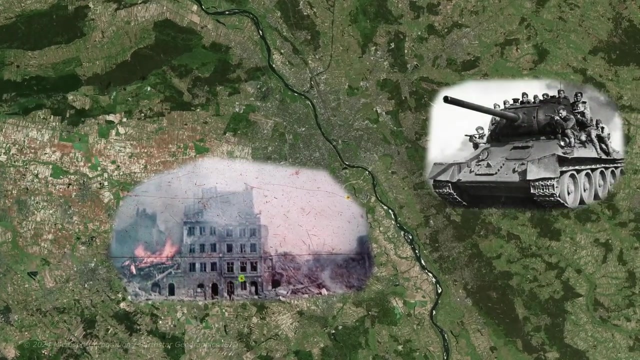 and executed them in the Katienmeister. The Polish set up an underground state to continue the fight and eventually rose up in armed rebellion in the Warsaw Uprising. The Soviets were now fighting the Germans and moving towards Warsaw. They decided to wait on the eastern side of the city. 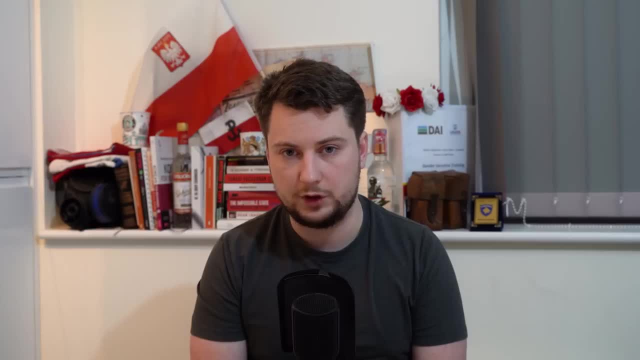 and watch as the Polish resistance were crushed F in the chat boys. The Soviets wanted a Polish puppet state, not an independent Poland. So after the war, that's what they enforced. The Germans were forced to leave Poland and the Germans were forced to. 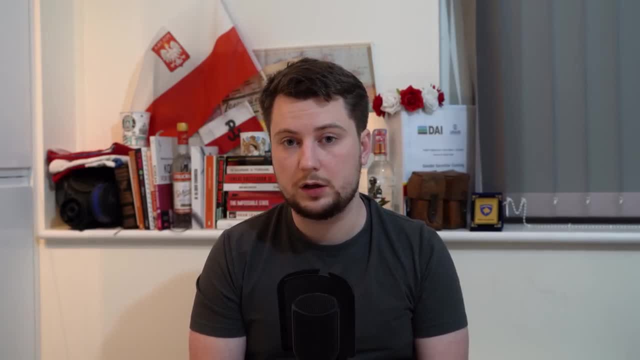 leave Poland. I found a common view in Poland being that we, as the British, betrayed the Polish in this moment, because we started the second world war on the basis of defending Poland from the Germans and by the end of it, they'd been turned into a puppet state of the Soviets. 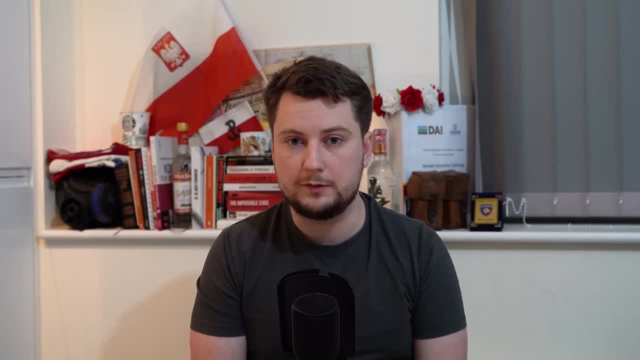 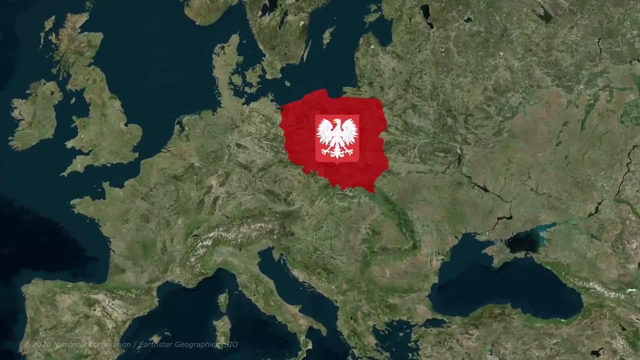 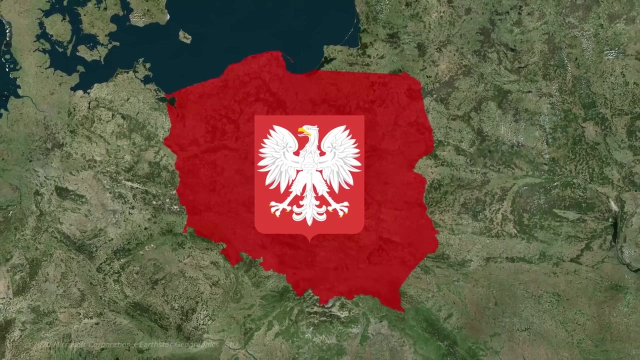 Now, I concede sympathy in this viewpoint, but frankly, beating the Germans cost us literally everything, so there was nothing we could do. But for the Poles this meant the fight was not over and Poland was not yet lost. They resisted the Soviet occupation as much as they could, and after a Pole became the Pope- 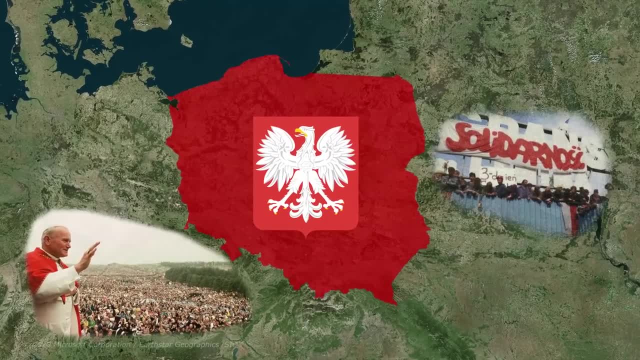 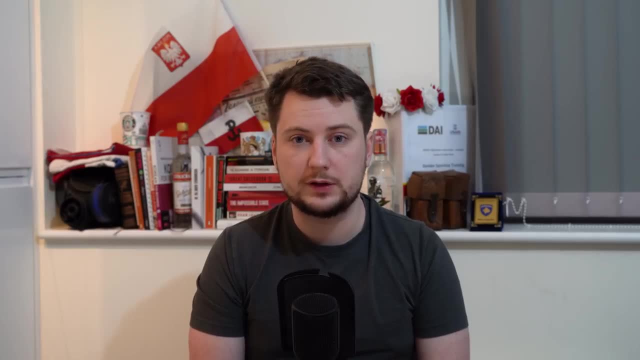 and visited Poland, the Solidarity movement was established and ultimately led to the liberation of the country from communism. This is the moment for Poland in which they consider occupation to have ended. From 1939 to 1989, 50 years of National, Socialist and Soviet occupation. 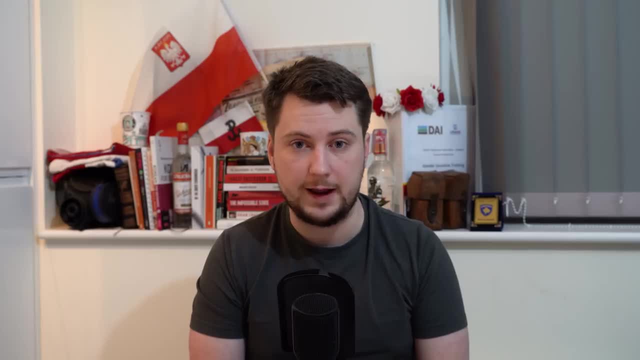 So naturally Polish politics is very anti-Nazi and very anti-Nazis. There are other points to look at, but in the end they are anti-communists. But back to Polish Independence Day. The government does put on a show in a celebration. 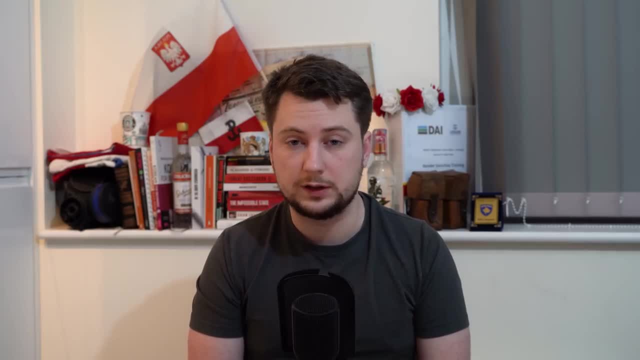 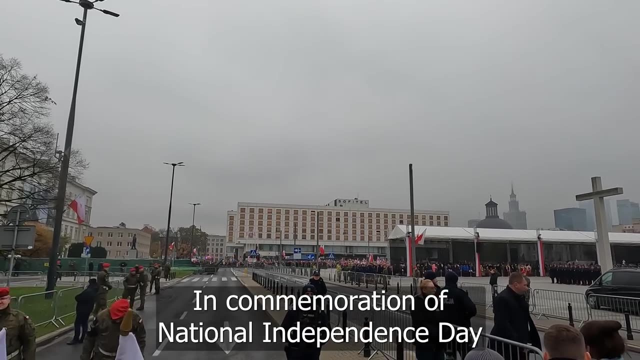 of Independence Day and it's very interesting. I did go to see it. POLE, YOU ARE GOING TO SEE AN INDIPENDENT SUBJECT. Pozoddziały skoci. Szanowni Państwo, Przemówienie z okazji Narodowego Święta Niepodległości. 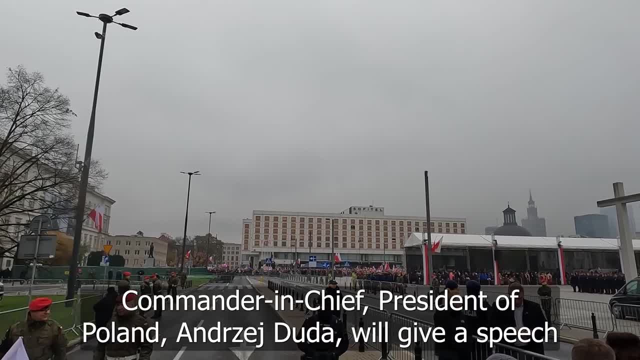 wygłosi Prezydent Rzeczypospolitej Polskiej Zwierzchnik Sił Zbrojnych. pan Andrzej Duda Walany na kolana wstawał za każdym razem. 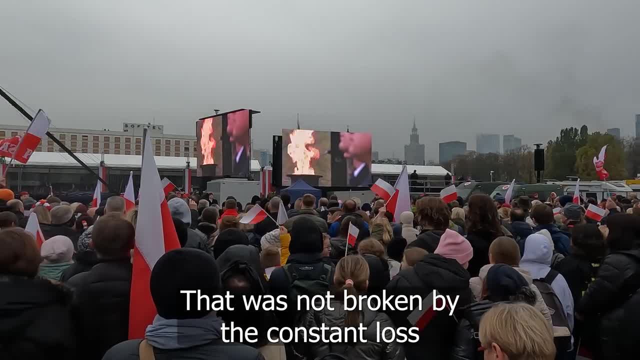 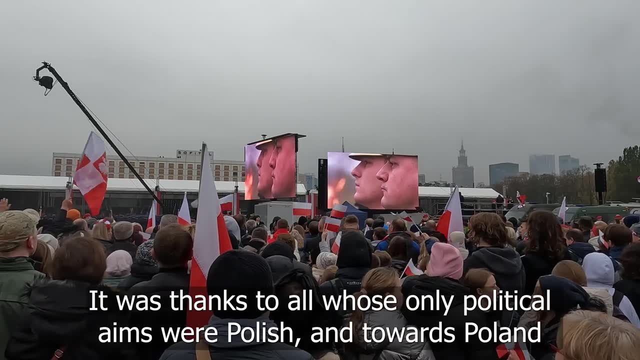 który nie załamywał się tym że ginęli koledze, and they kept on telling the British to join in the war. Zそう the next one who went forward, believing that he would regain his state. it was thanks to. 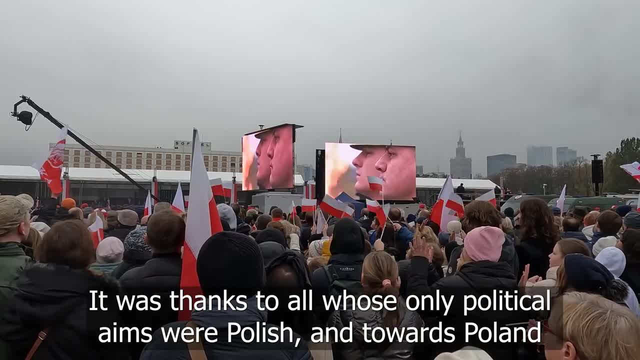 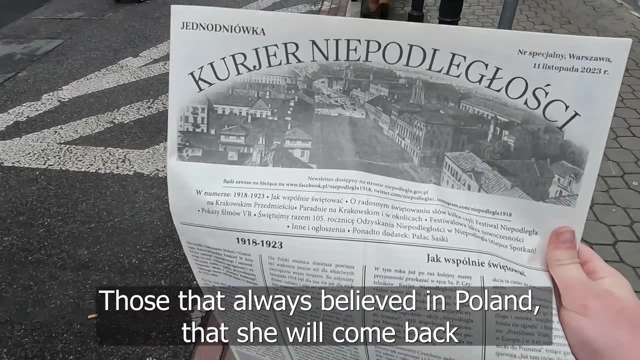 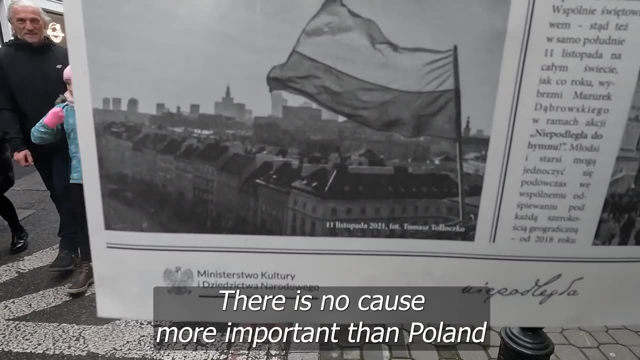 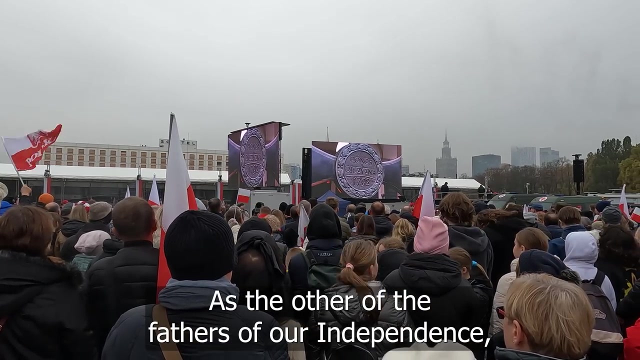 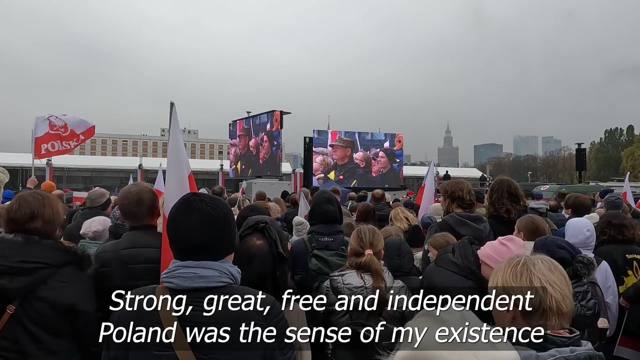 the fact that all those who then led the Polish politics and to Poland- they firmly believed in this Poland, that it would return, said vincenti vitos. there is no matter more important than Poland, said the second from the fathers of our independence, ignacy jan paderewski: strong, great, free, independent. 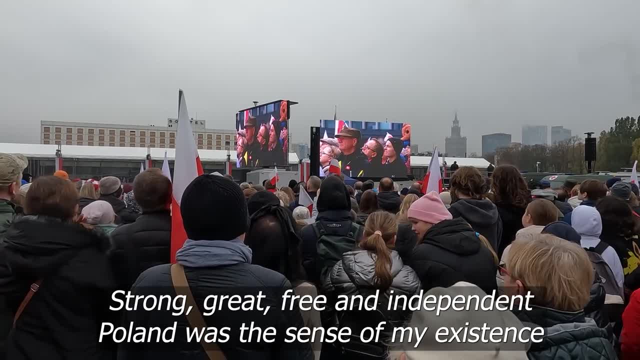 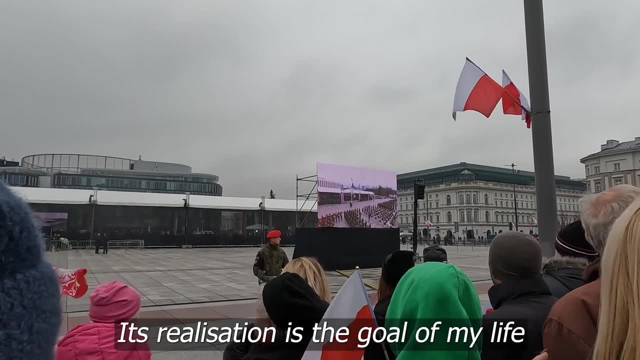 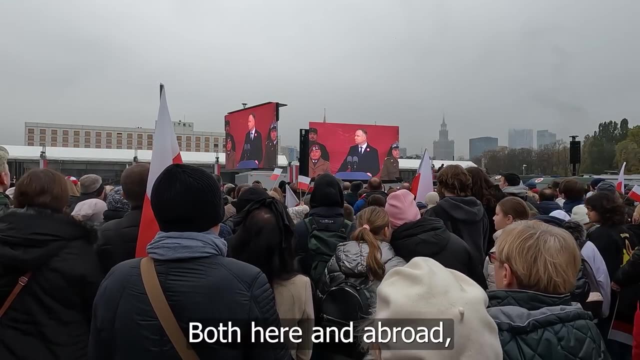 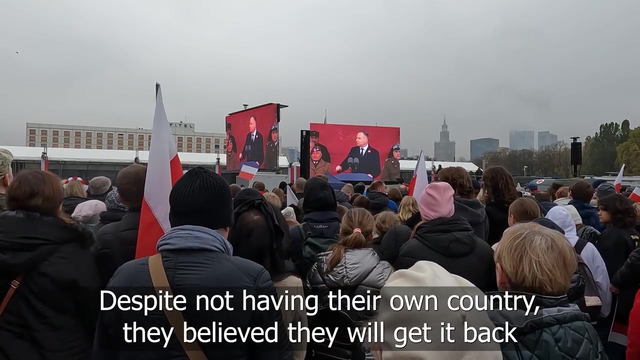 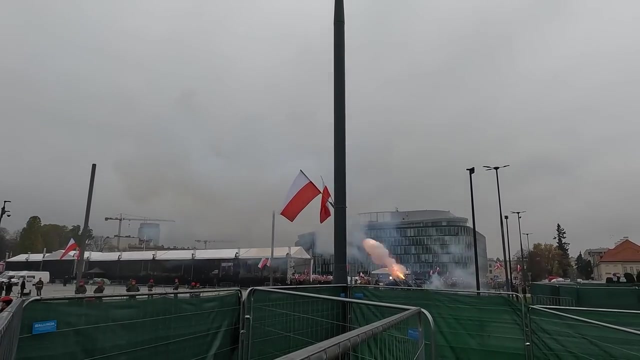 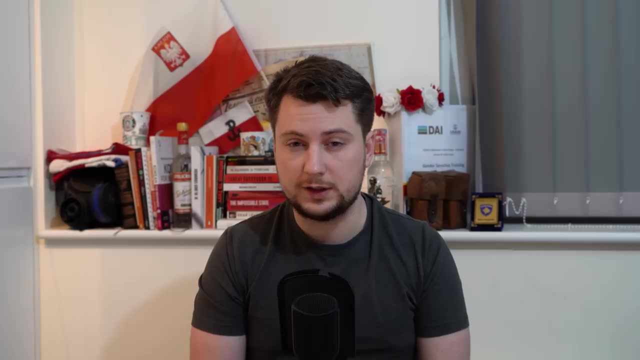 poland was the essence of my existence. its realization is the goal of my life. they believed, But it's not what attracted international attention. The international attention of Polish Independence Day is on the march, And the march's history is very interesting. From what I can understand, it started out as basically some angry lads who were upset. 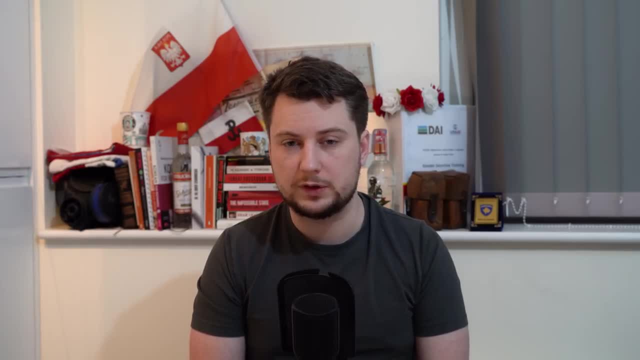 about the way Polish society was going and wanted to make their voices heard, so organised a march in central Warsaw. Now, some socialists decided that they wanted to oppose this march, declaring the marches as far-right, and so turned up calling themselves Antifa, and scuffles quickly broke out. 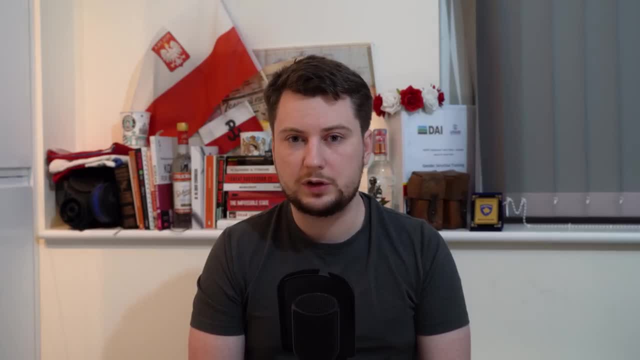 But this is what exploded the event, Because there were socialists trying to suppress a Polish Independence Day march. given the history of Poland, this didn't look very good, And what happened is that the popularity of the march skyrocketed and ever since has. 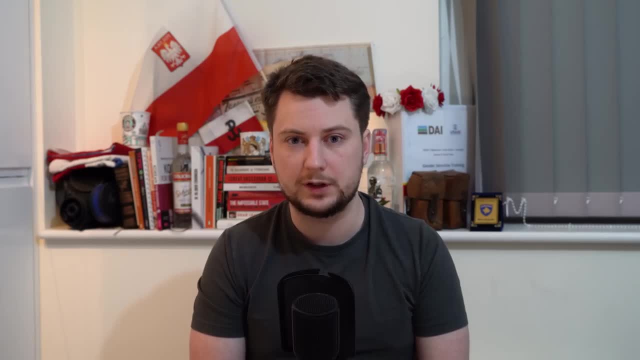 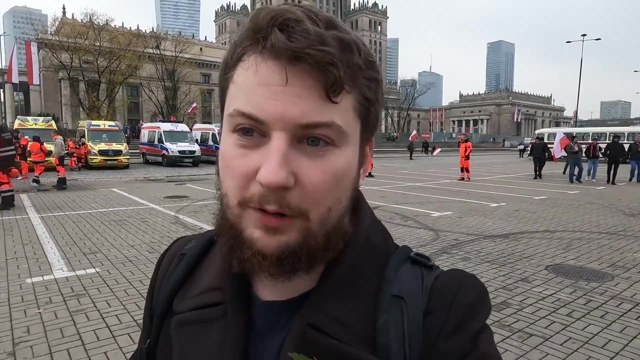 attracted thousands, if not tens of thousands, of people every single year. Also, one of the nice things about this march organised by the Nationalists is that you don't need to speak Polish. You can get the message Pretty quickly as to what this is about. 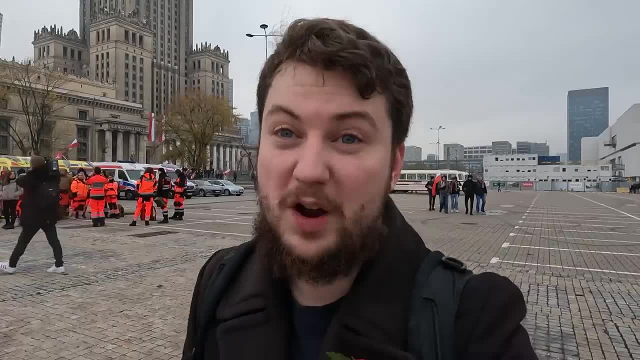 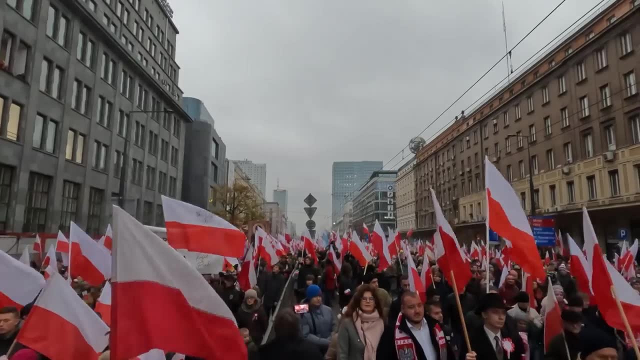 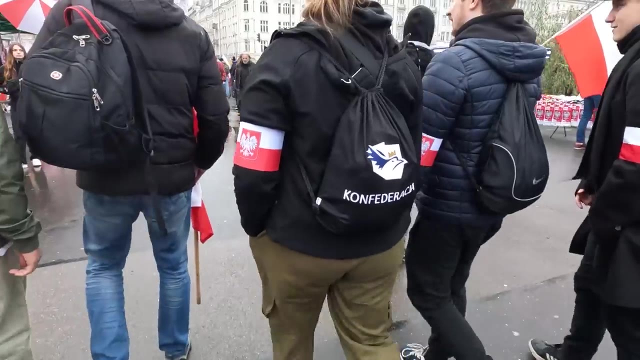 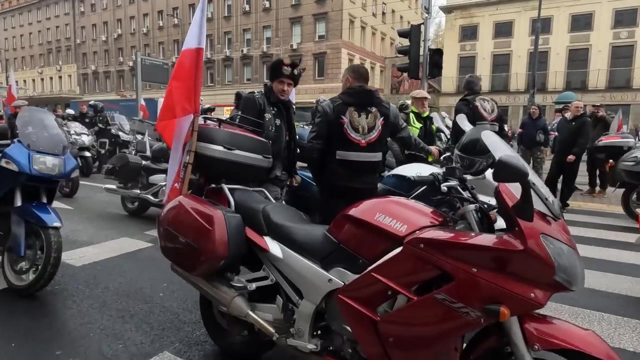 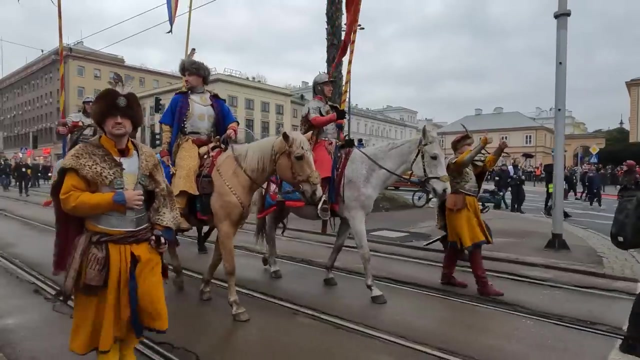 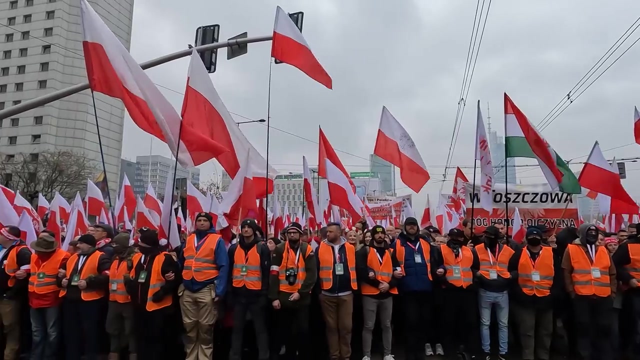 You can be an illiterate serf and still understand what this is about, which is basically what I am, Because I don't speak Polish Or read it. It's a hey-ho Time to be a serf, beneficially. 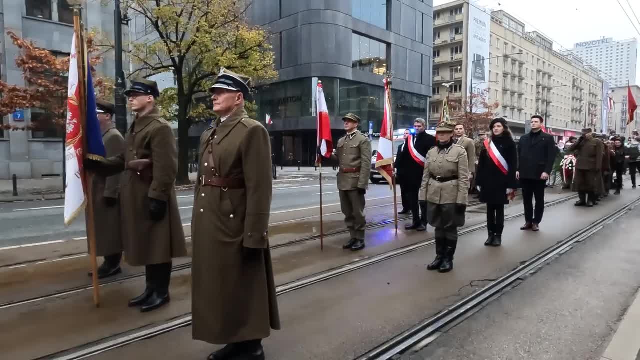 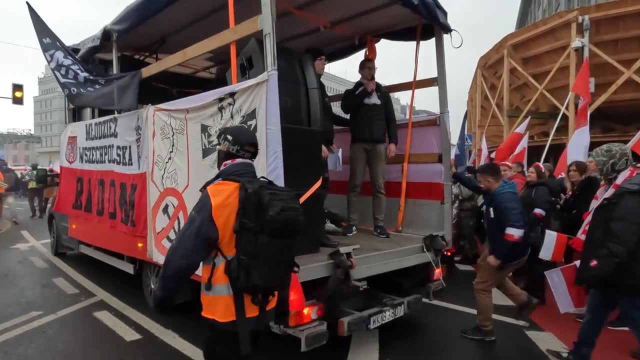 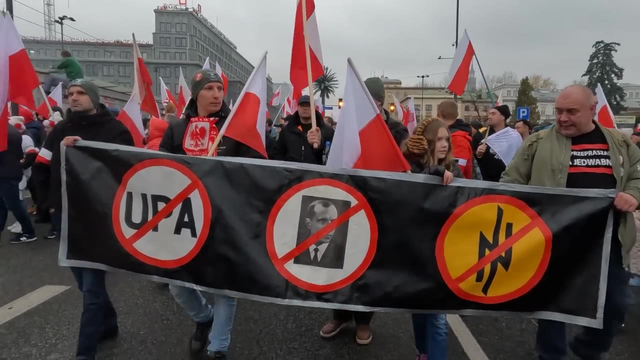 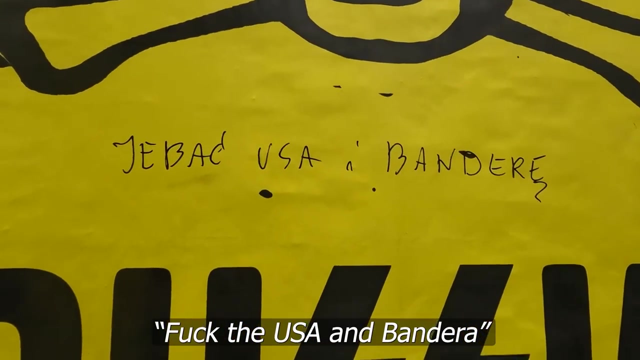 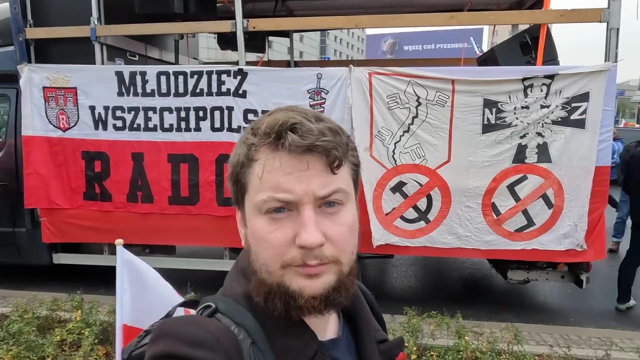 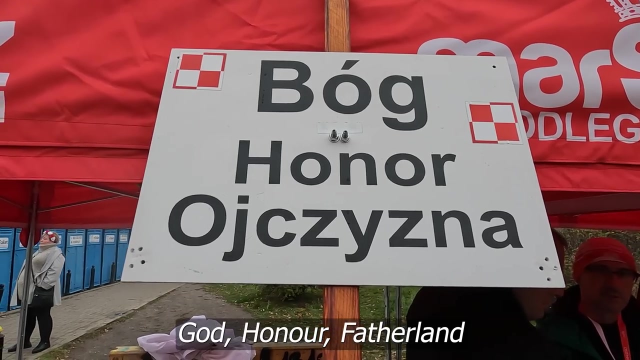 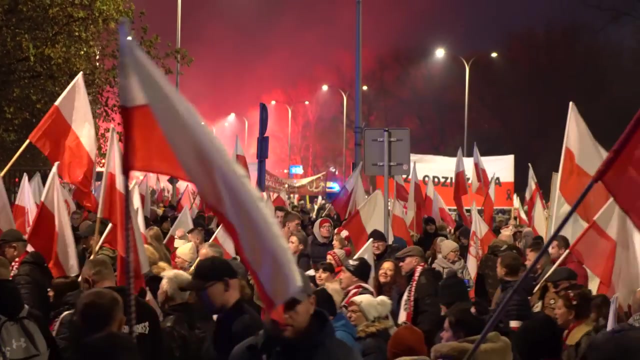 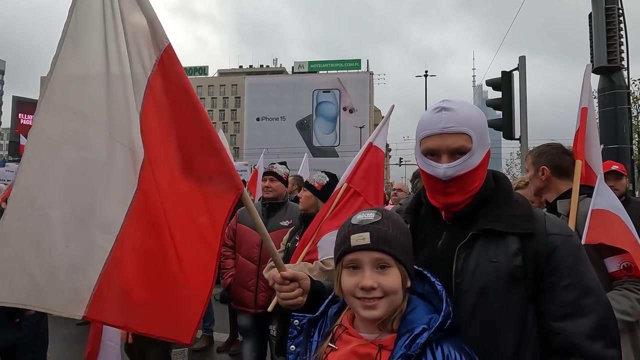 See you later. Bye, guitar solo. I was actually lucky enough to meet Christoph Bozak, who was one of those angry lads in the 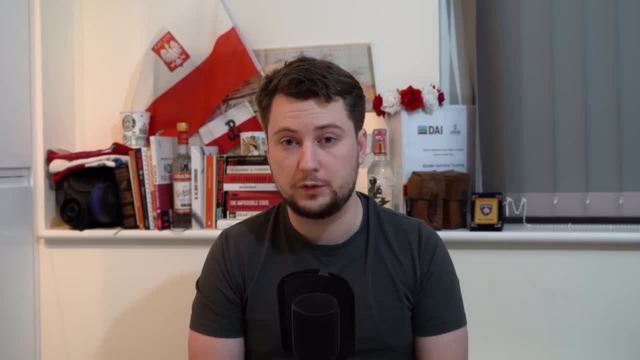 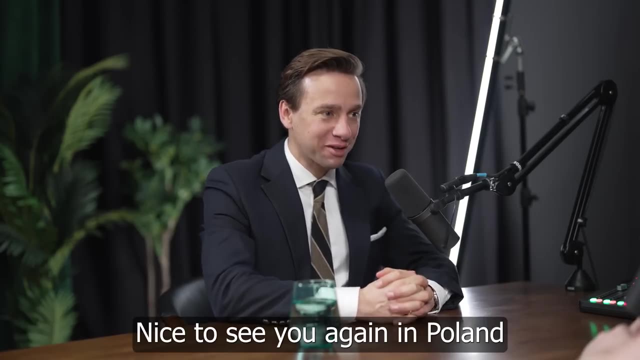 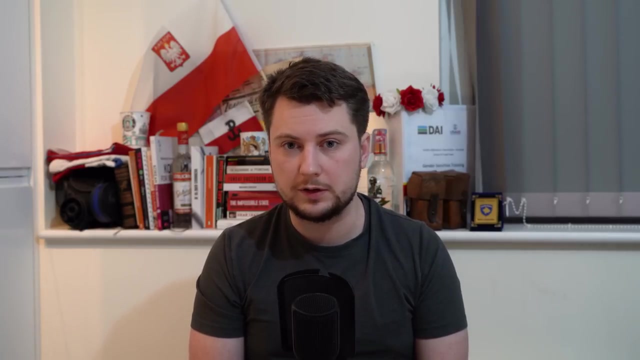 beginning and I got to interview him at Visegrad24 studio, who happened to be friends and very kindly let me use their studio for it And thank you for joining me. Nice to see you again. So I think I'm going to cut in segments from Christoph where they make sense. It's a bit weird that my holidays now. 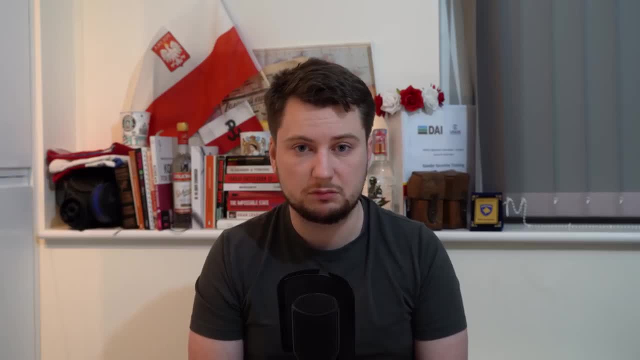 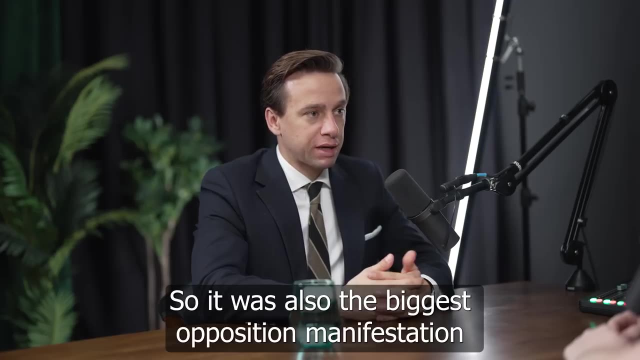 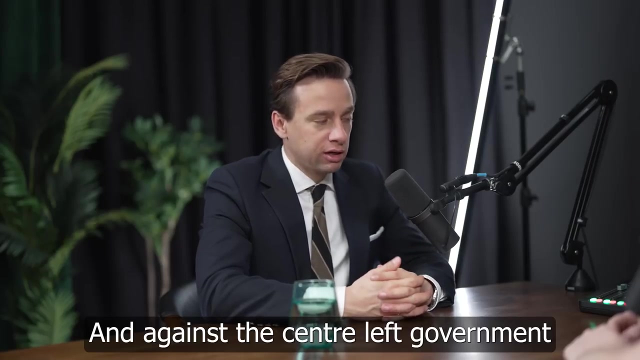 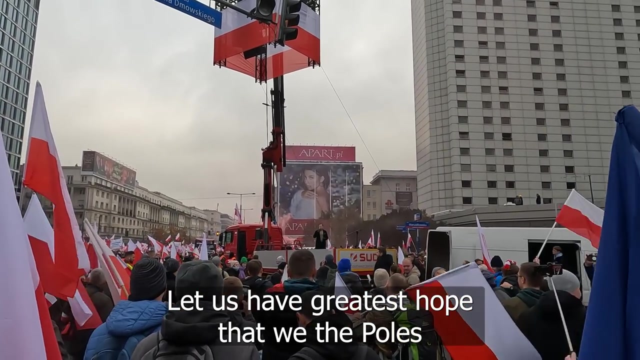 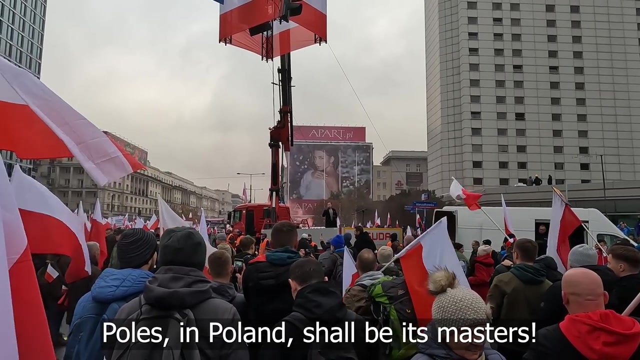 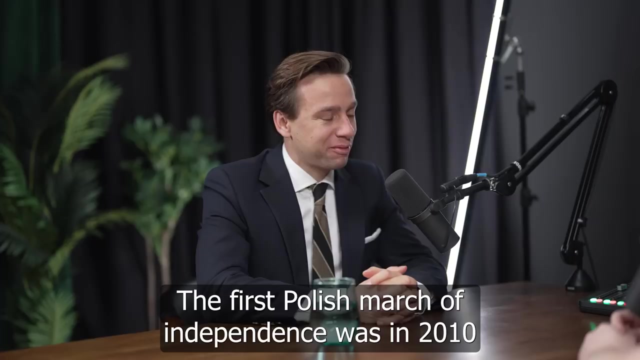 consist of interviewing politicians, but it's good fun. It started during progressive government of Civic Platform, So it was also a biggest opposition manifestation against political correctness and against center-left government. First Polish March of Independence was in 2010.. And they tried to physically block it And they 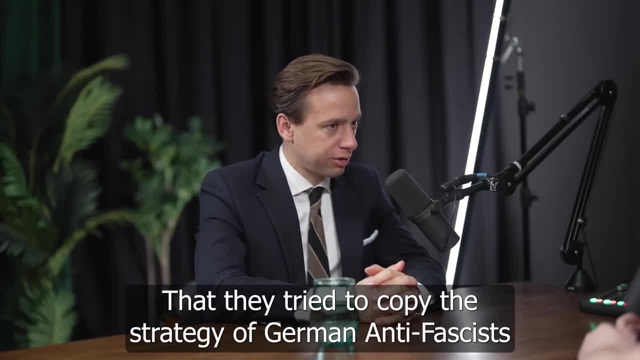 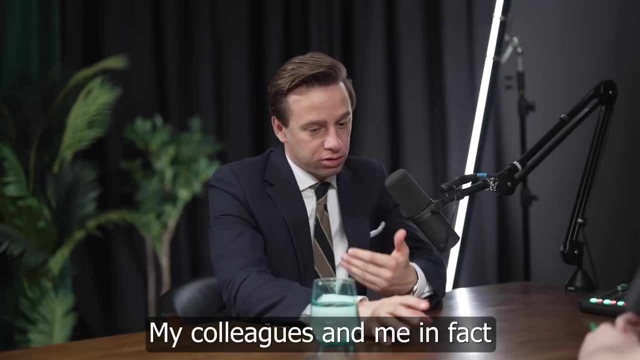 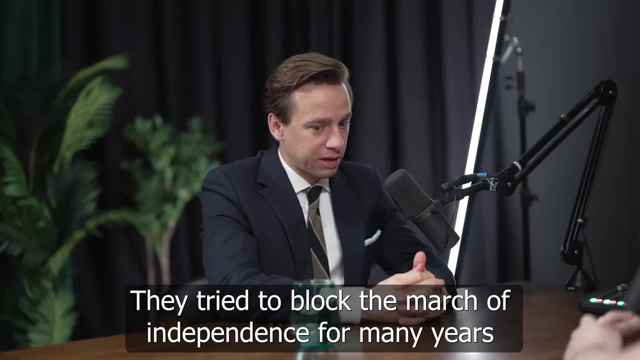 openly said that they tried to copy the strategy of German antifascists. So they branded organizers- my colleagues and me, in fact- as Nazis, which was 100%. They tried to block March of Independence for many years, but they didn't succeed, And since maybe seven or eight years they don't try to block. 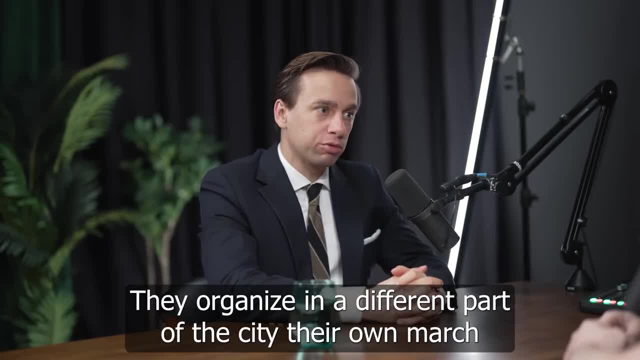 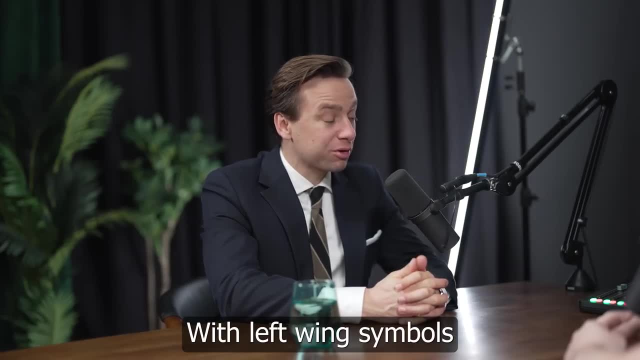 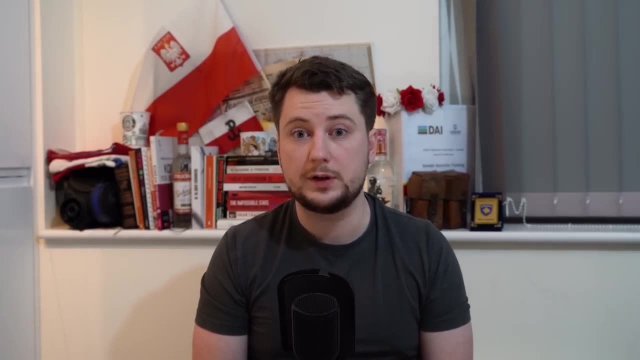 They organize, in a different part of the city, their own March: small, without Polish flags, with left-wing symbols. With the March becoming so large and infamous, it started to attract political attention not only from the major parties in Poland, but also internationally, and has now become a meeting point for national and international meetings. 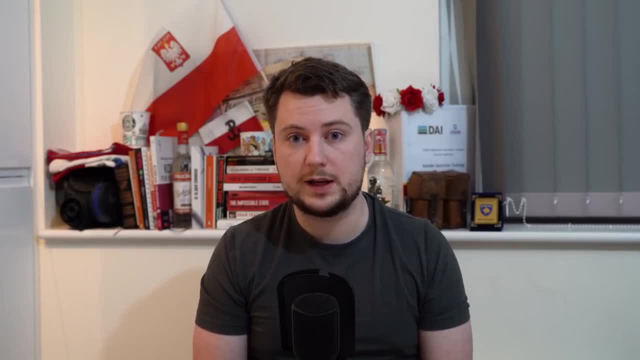 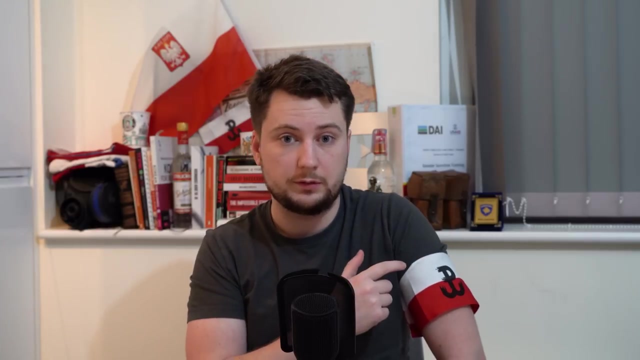 But the vast majority of the attendees are just Polish patriots of all kinds. The main thing that everyone does is buy themselves Polish flags. Polish girls buy themselves Polish flag-coloured hairbands, But what everyone does is get themselves Polish armbands, the same style that were used during the Warsaw Uprising. 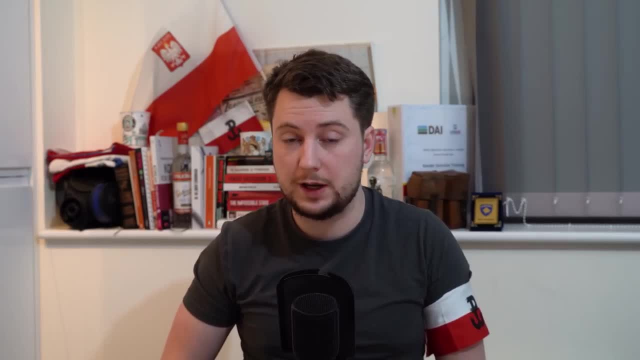 And I did manage to bring a few back, so those will be the only items I have for sale this time around For people who don't know. I like to bring back things and sell them. I sell them from the various trips to help fund them and it gives you something in return for subscribing to help keep the financing coming to do these things. 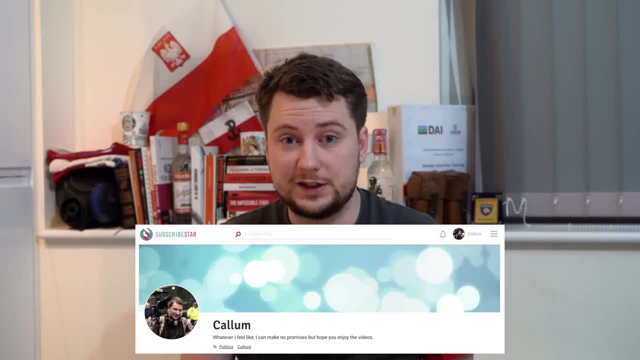 So if you'd like to do that, you can go over to Subscribestar. ask me if they're still in stock and if yes, I will be able to sell you one. Otherwise, you can always just subscribe to keep the videos coming or purchase some of the old stuff from the old trips. 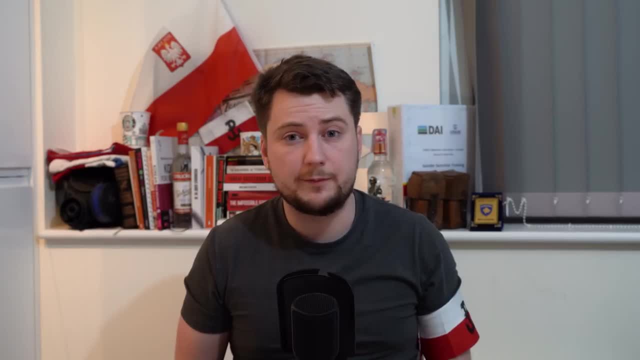 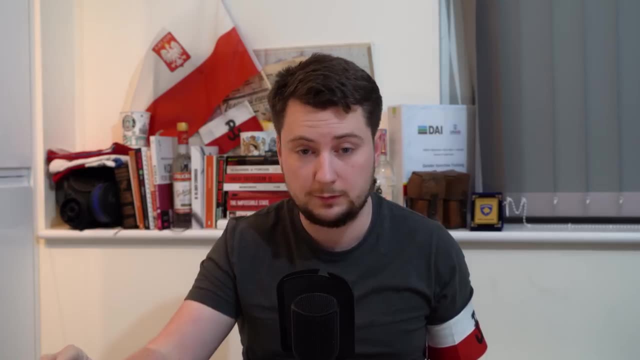 And again, thank you to everyone who has you make this possible And, for the time being, everyone who subscribes gets access not only to the Private Members Club on Discord, but also ten Soviet rubles for free, Because I still have plenty to go. 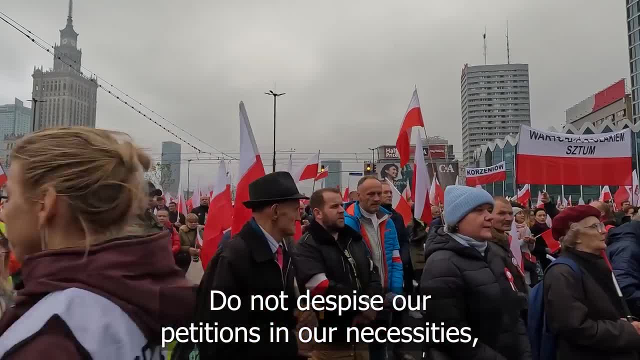 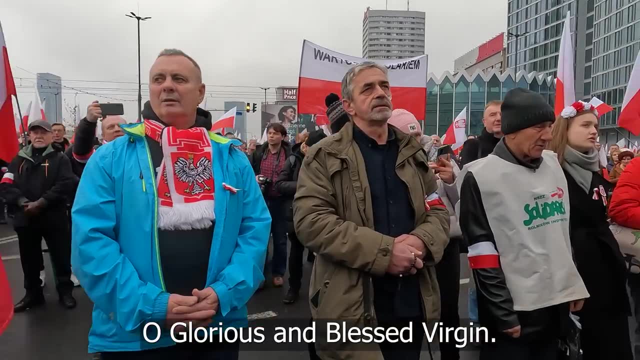 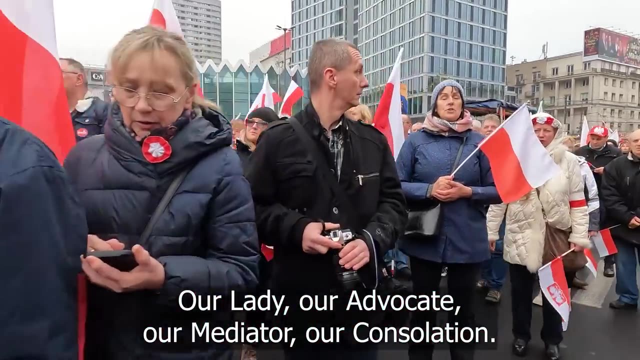 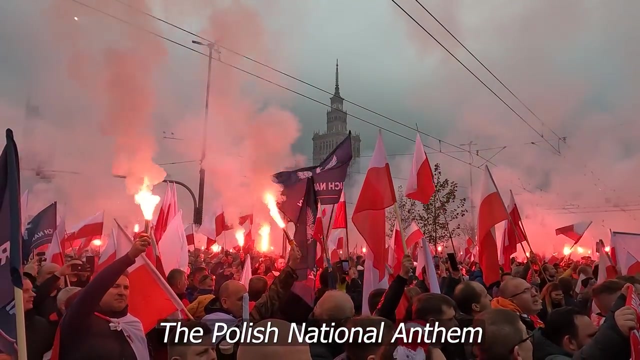 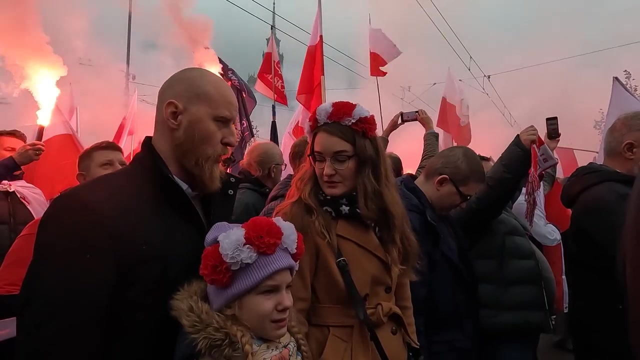 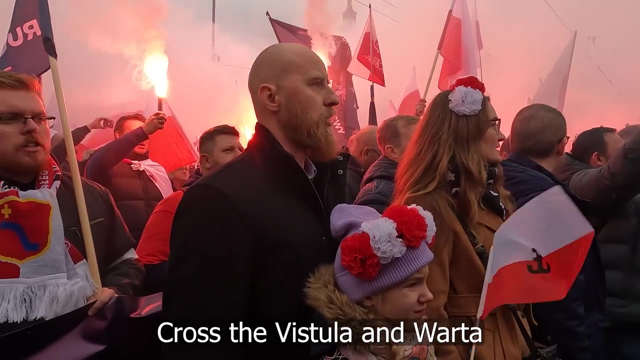 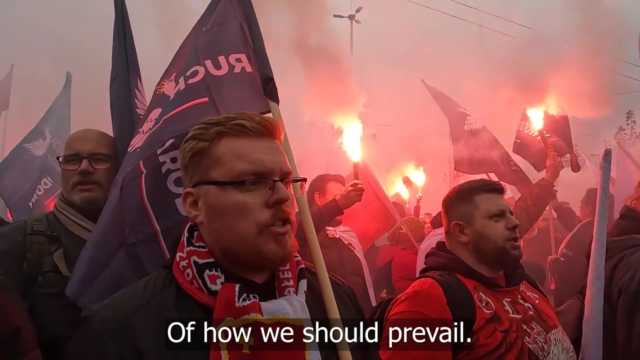 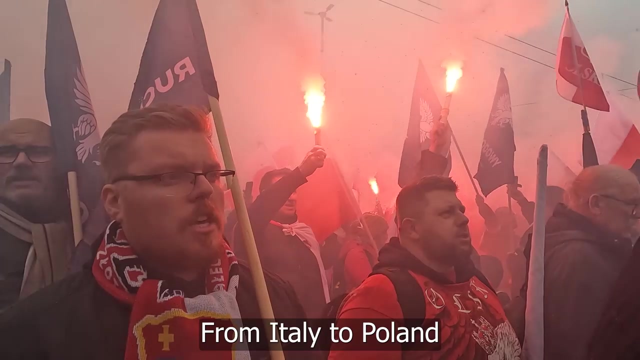 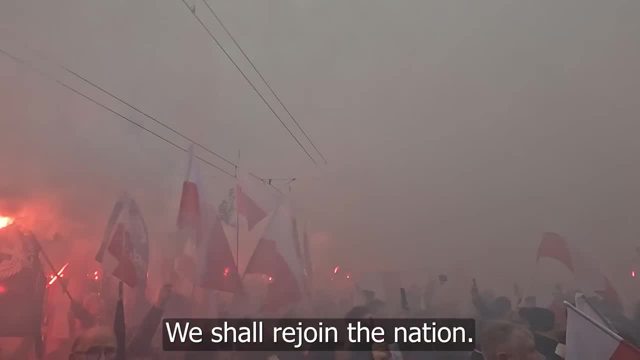 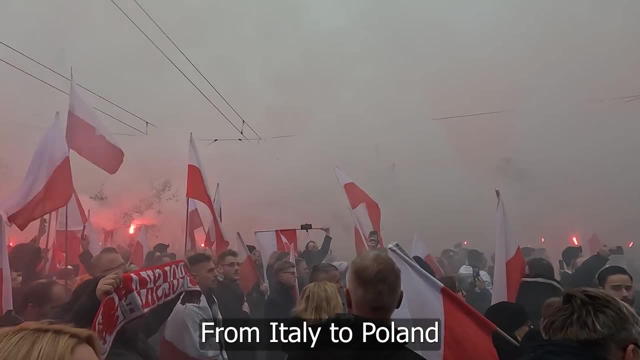 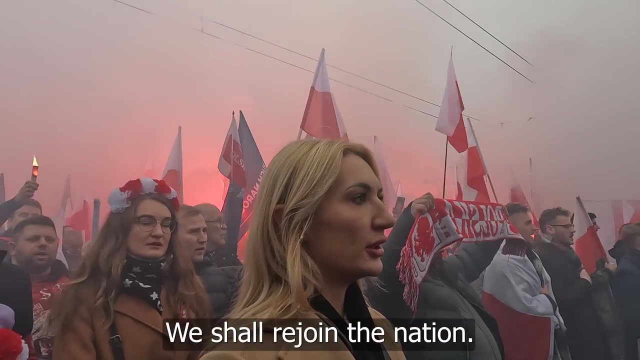 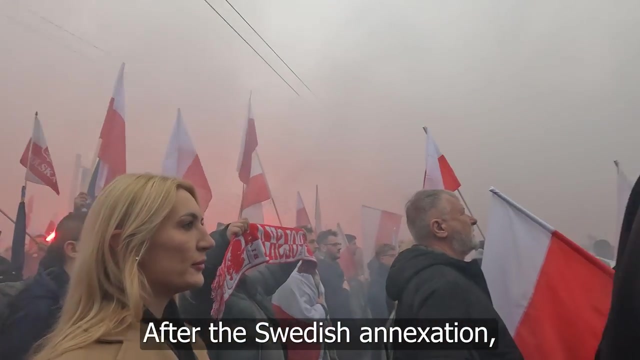 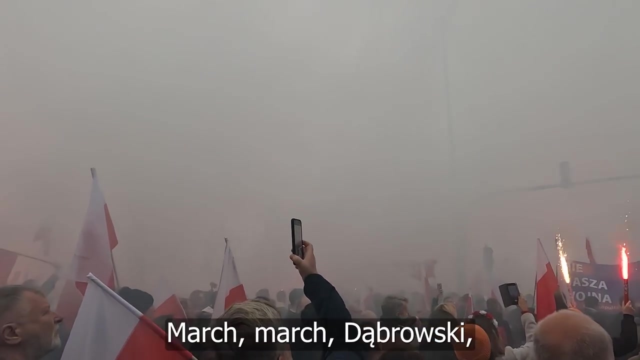 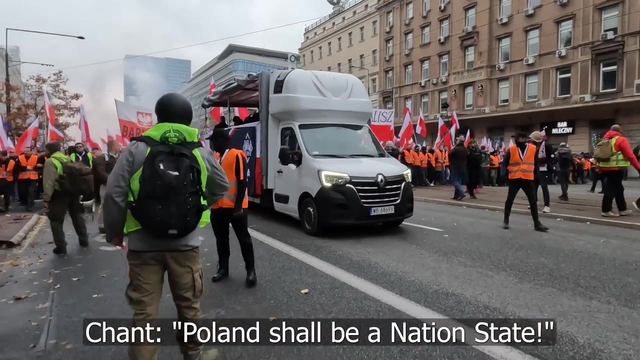 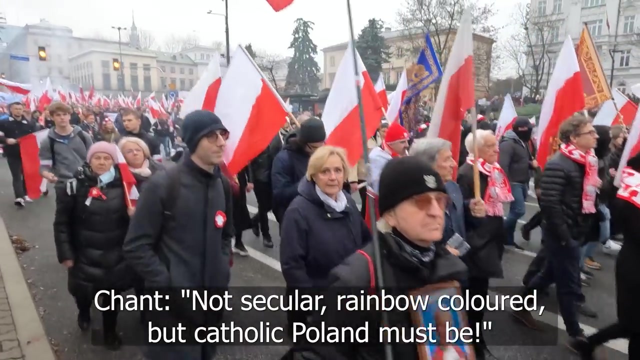 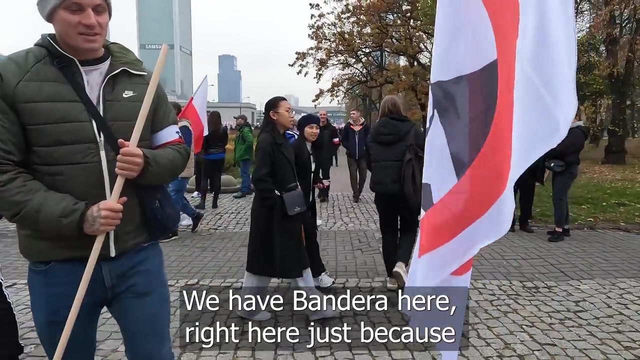 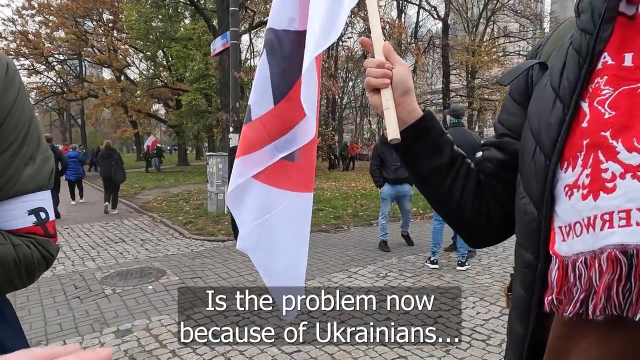 Bye, Bye, Bye. why do you have bandera? you got bandera here, right here, just because we hate him. he killed poles and jews. yes, of course. obviously is the problem now because of ukrainians. yes, they come to poland and still like him. yes, yes, yes, okay he, he is their hero. you know he have 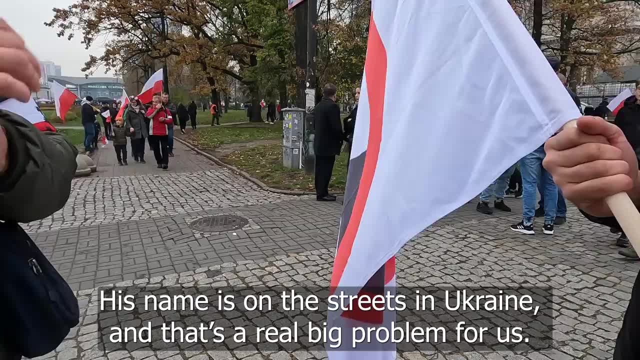 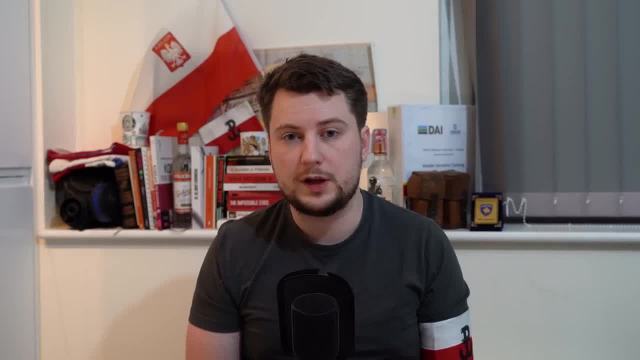 monuments in cities. his name is on the streets in ukraine and that's a real big problem for us. but the main focus for most international media was on a small group that turn up every single year, this one included of fascists and white nationalists, usually because this is something. 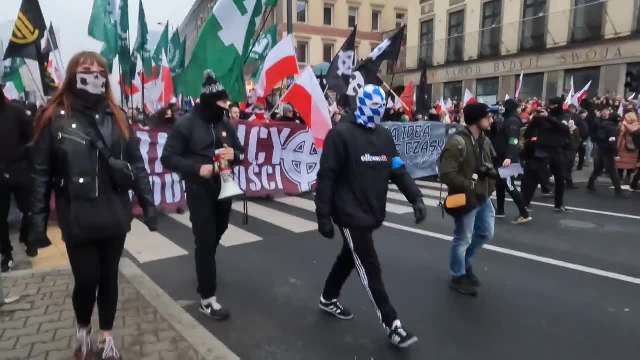 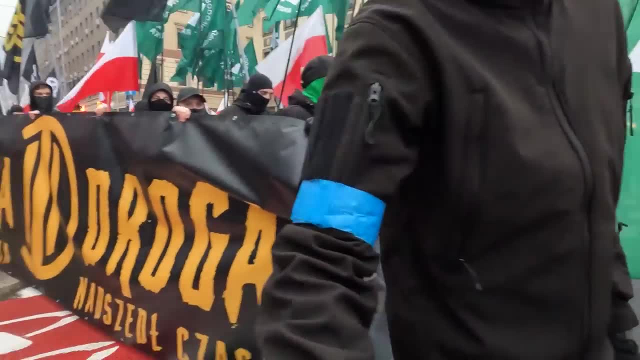 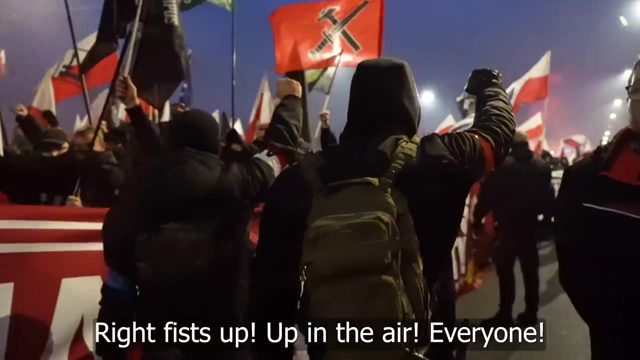 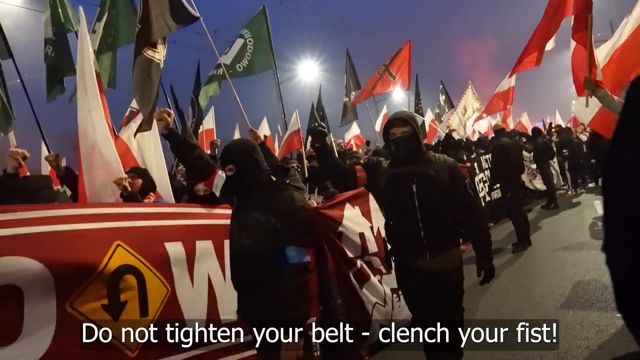 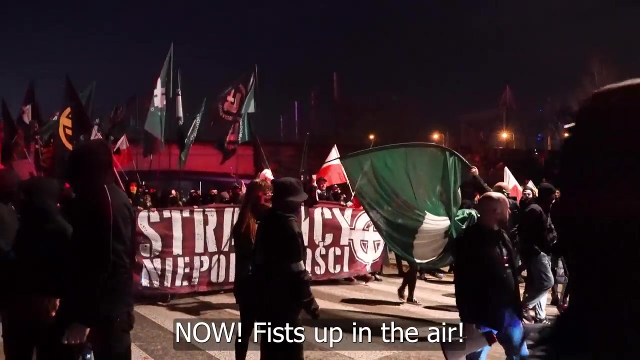 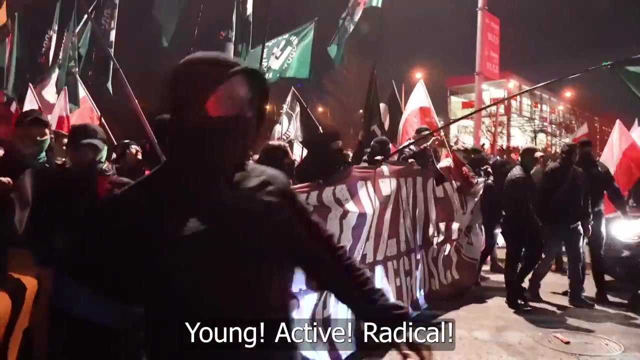 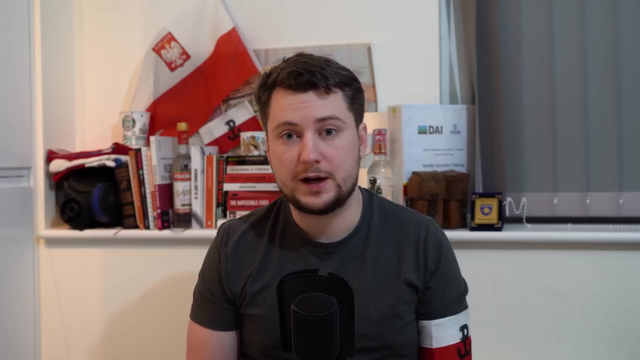 to shock their audiences with. these guys like to turn up in black with their faces covered, and keep organized to themselves in a block. they force people with cameras out and chant their slogans with the image they are giving off in mind. i did manage to speak to a couple of these people, which included a couple of americans. 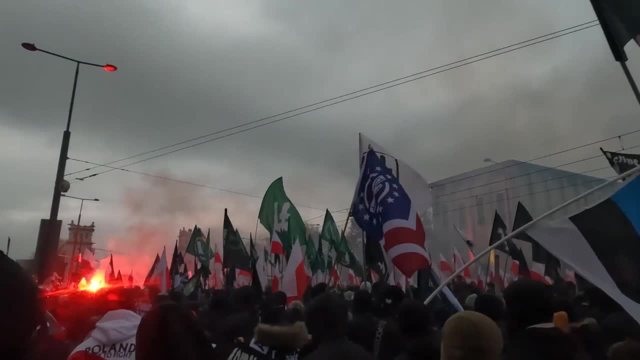 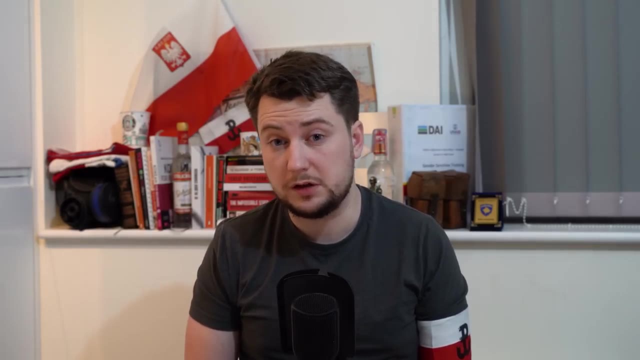 in fact, one of them was from the american group patriot front. so i went up to him and said: hello, my fellow fed, and he responded: ah yes, another fed. the rest of them, however, didn't seem to have much of a sense of humor and acted with hostility to any kind of questions. 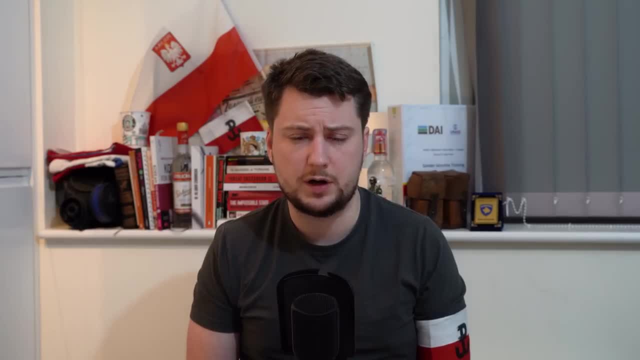 and most of them were not so hostile to any kind of questions and most of them were not hostile to any kind of questions and most of them were not so hostile to any kind of questions. but interestingly, this aspect of the march seems to be the most international, with european 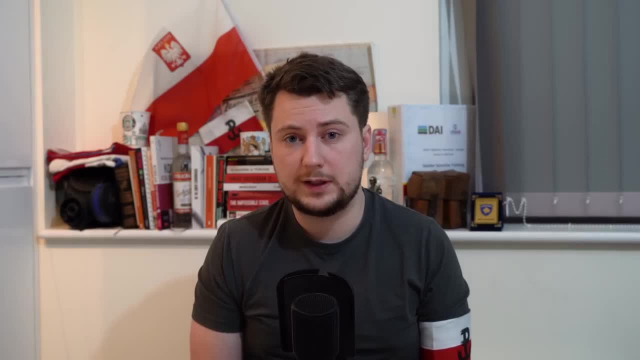 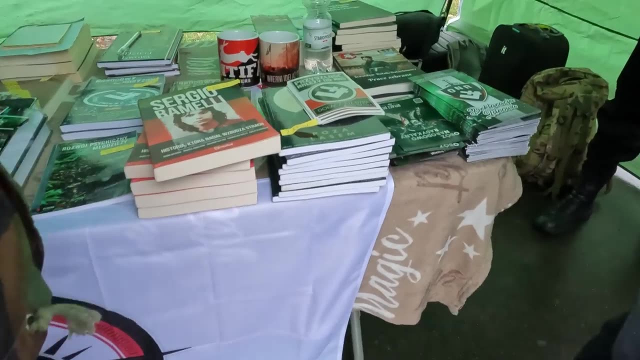 fascists from all types turning up. if you think i'm being a bit of a silly journo by using that word, i don't believe i am one of the groups even called themselves the syndicalish socialist alternative. they seemed like the kind of people who would read an awful lot. 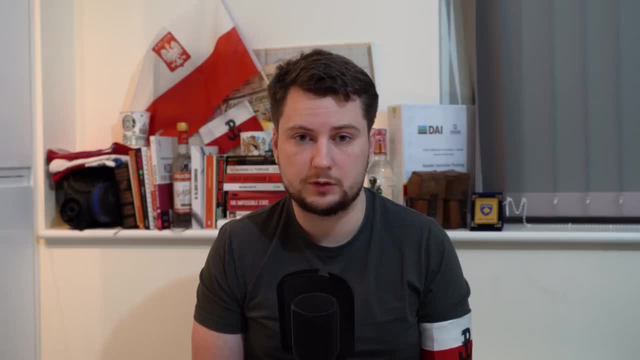 of political theory, although most of them were as hostile to me as socialists are in the uk. it was kind of interesting to see genuine fascists in the flesh in the anglosphere, the uk. this is, of course, incredibly rare. it was always like that on the march of independence. 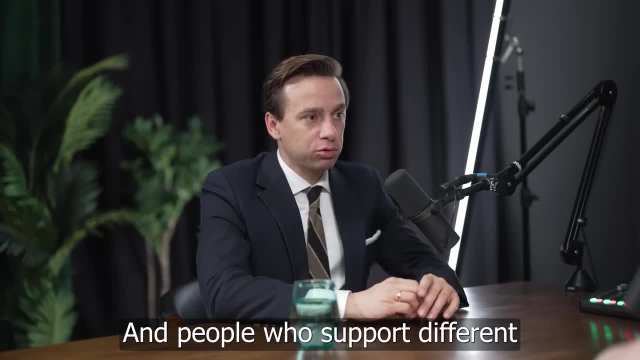 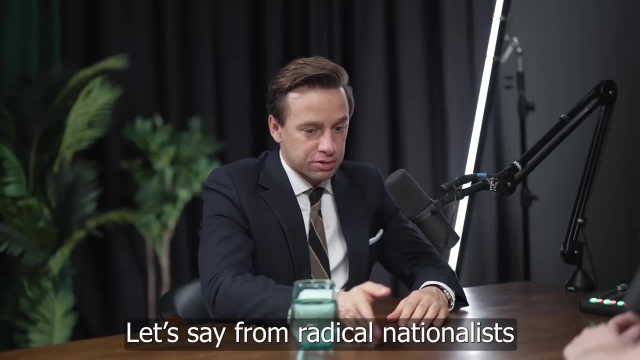 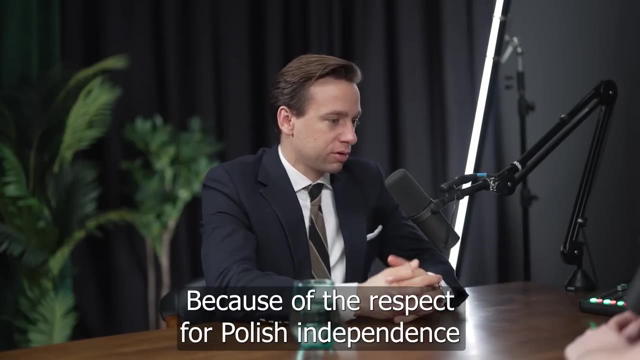 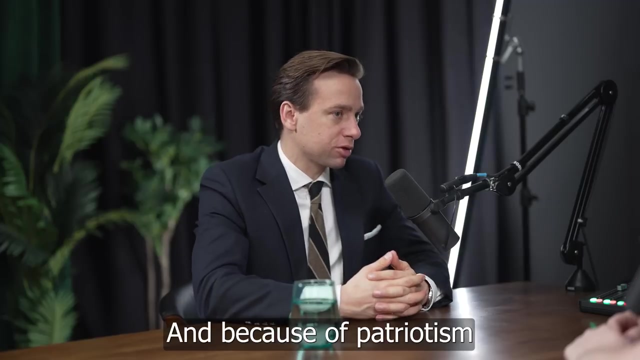 that many different groups with different views and people who support different football clubs or different political parties, let's say, from radical nationalists to people who support law and justice. they march together because of the respect for polish independence and polish state and polish tradition, history, heritage and because of patriotism. i think it's good. 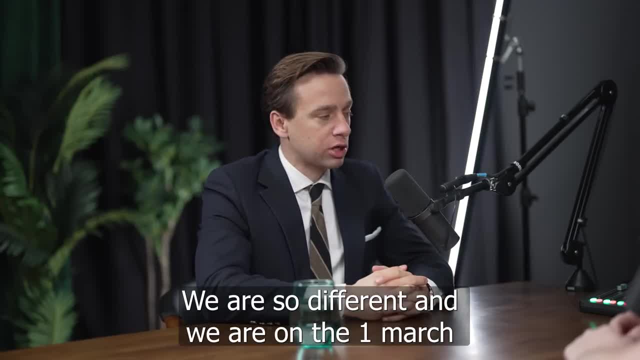 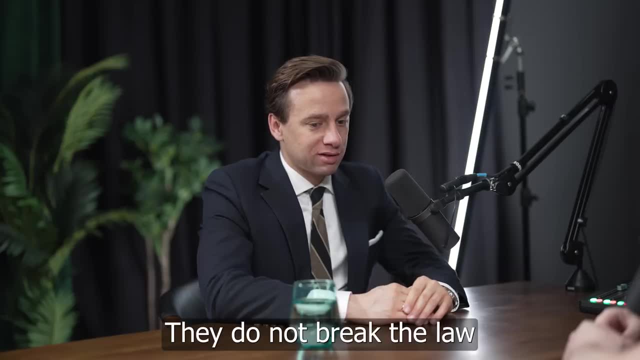 that we are so different and we are on the one march and we accept that situation. they have their own views. they would like to express their views. they do not break the law, so they have the right to be there. they are polish patriots. i do not agree with them on many levels. they probably 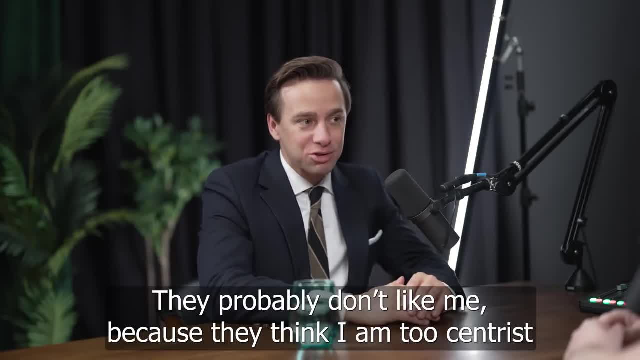 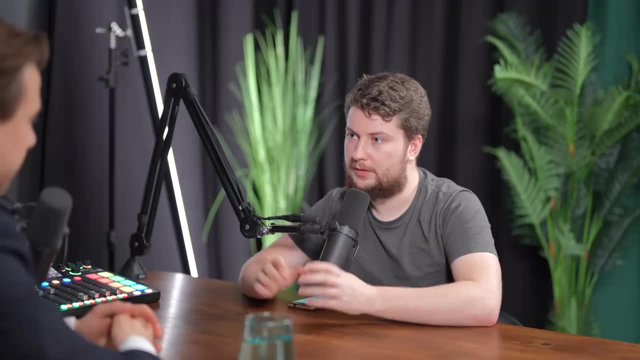 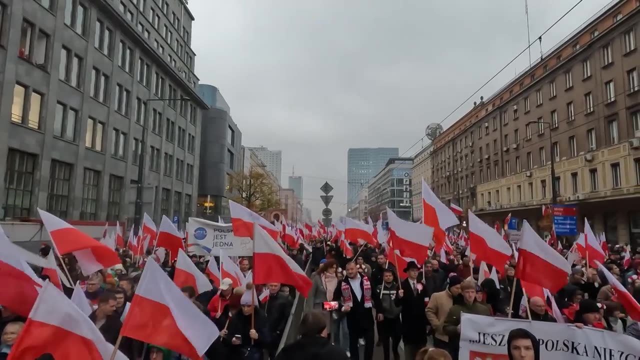 don't like me because they think that i'm too centrist. they even had some slogans against us as a confederation this year. but that level of political diversity i mean. i saw people, for example, all the way from being completely normal centrist polish flag wavers to people who were 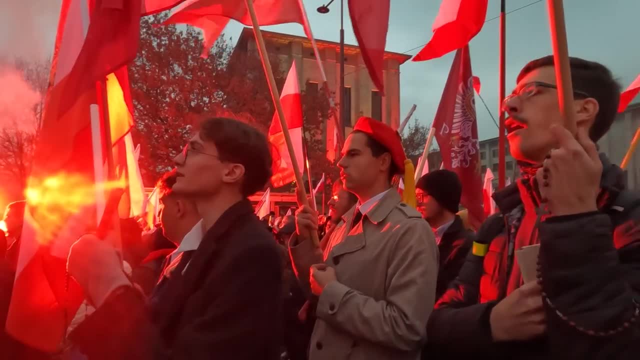 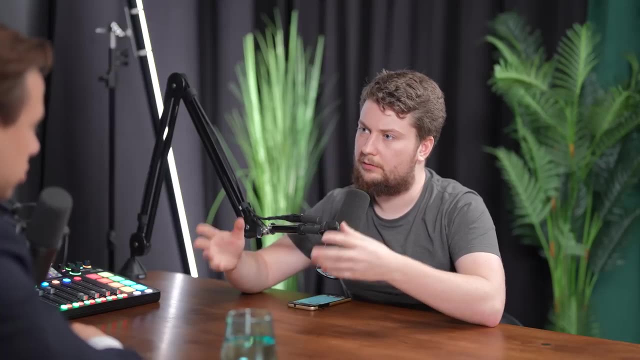 there with anti-azof banners, catholic nationalists, and then at the black block i'd find people even with, like the black sun- there was one guy with that, so is this is the reason this is the case, this massive political diversity? is it because it's a march open to everyone and therefore, if 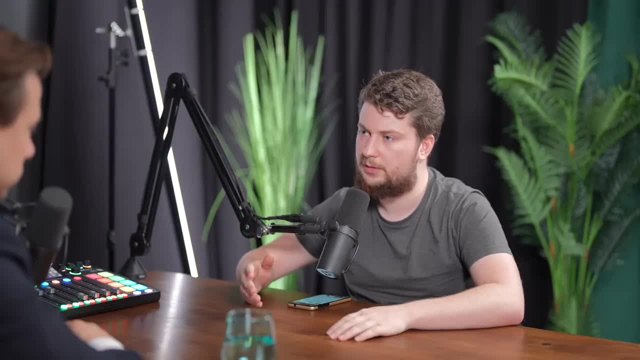 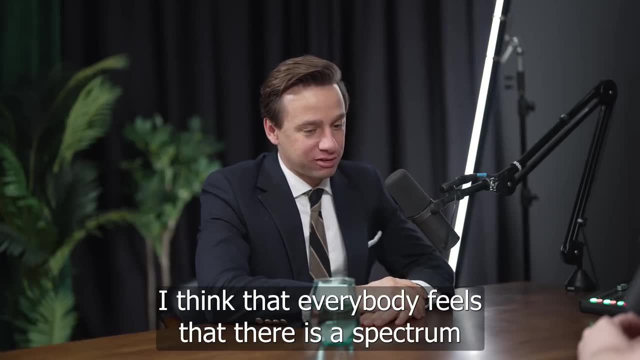 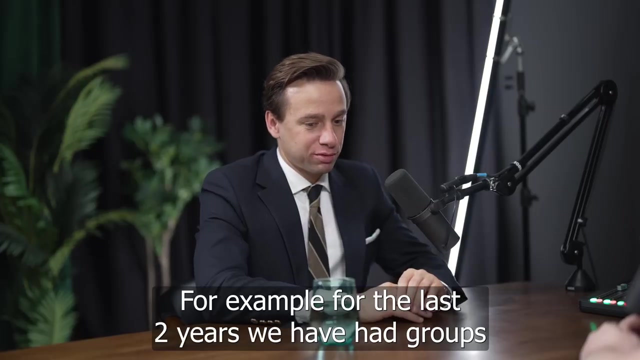 you support poland, even if you're a socialist or communist, they would be allowed to be there. good question, i i don't think so. i think that everybody feels that there is a spectrum for polish patriots and we can argue on many issues, for example, last two or three years. 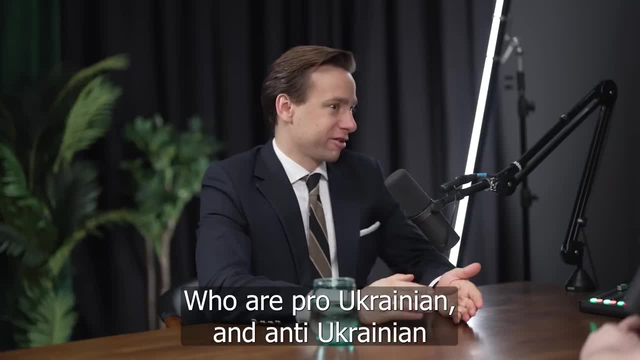 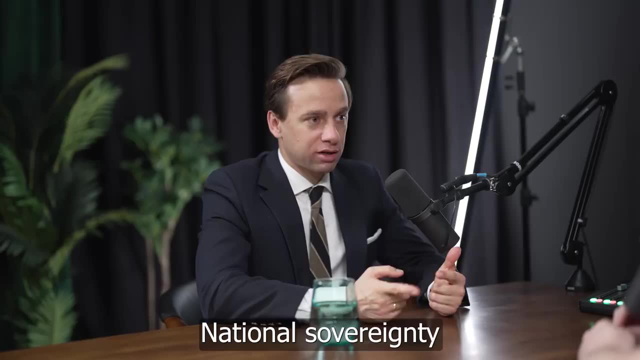 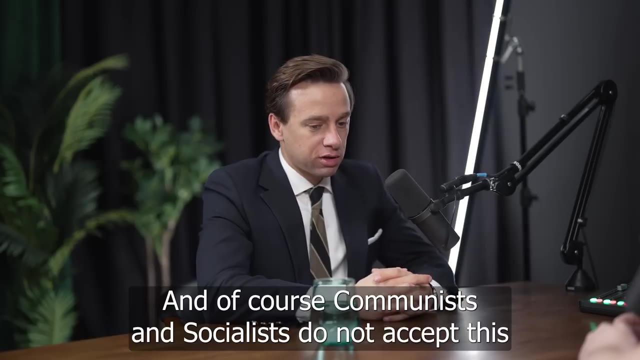 we had groups who are pro-ukrainian and who are anti-anti-ukrainian on some level, but you should accept basic values: polish independence, national sovereignty, respect for the tradition, respect for christian values. and, of course, communists and socialists do not accept this. and what is most, 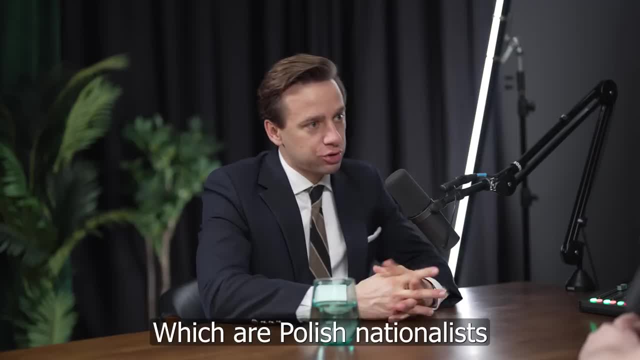 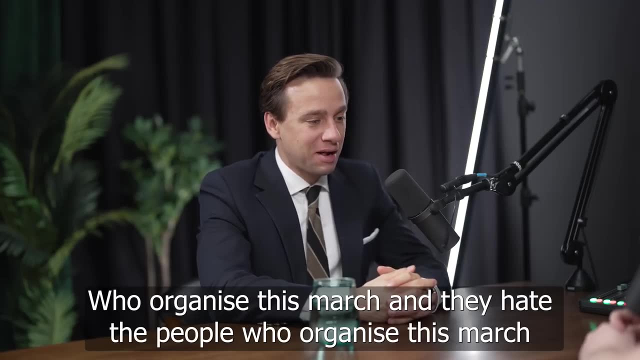 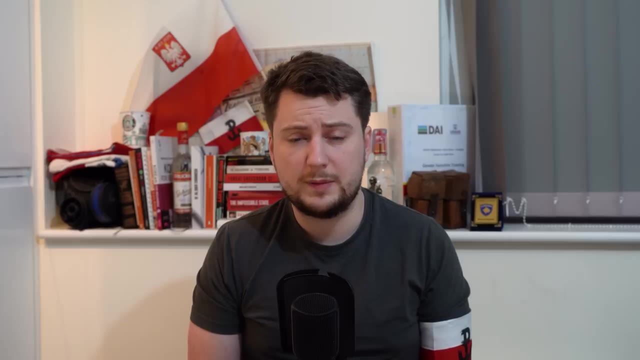 important. they do not accept the organizers, which are are polish nationalists who organize this march and they, they, they hate people who organize this march, so they will never come. but, as i mentioned, these guys are a really small part of the march. the main march is made up of just mass. 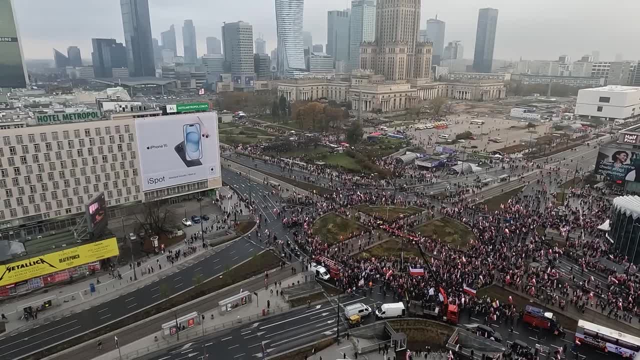 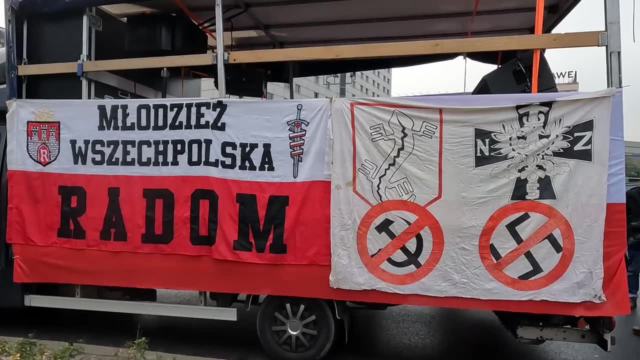 amounts of polish patriots from all kinds of groups. the vast majority of them are from the majority are random polish patriots who wave polish flags, but there are also polish reenactors, biker gangs, anti-socialists, anti-abortion, anti-eu types, anti-stephen bandera activists. 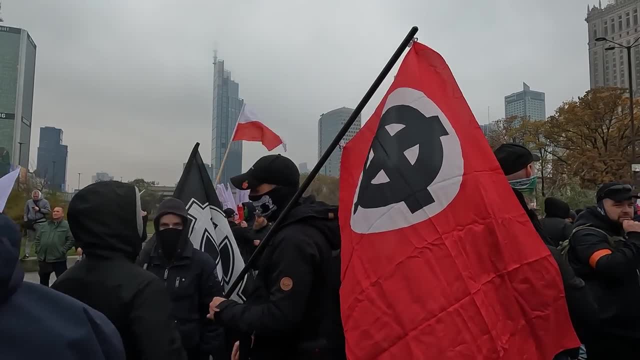 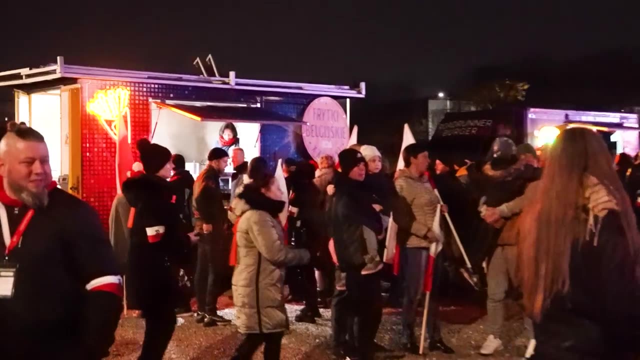 and then there are the polish fascists and white nationalists, the kind of people who think about the roman empire a lot. the whole thing ends near a football stadium with a stage show, street food, and is right next to the train station in case you want to get out of the cold. it's a strangely. 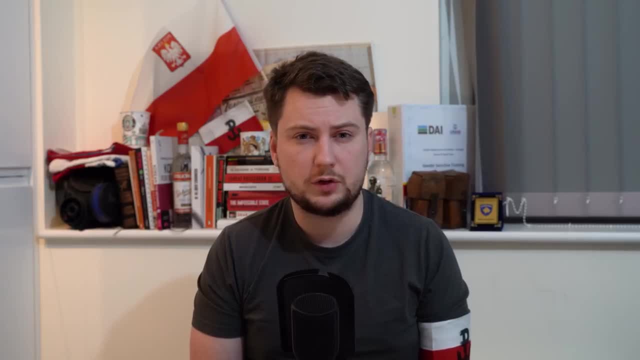 nice thing to have witnessed. i don't think i could ever say that i took part in this or can even take part. it felt instead like i was observing the polish right and how they interact with their independence. everyone was incredibly tolerant of each other, which might seem a strange thing to note, but the group isn't. 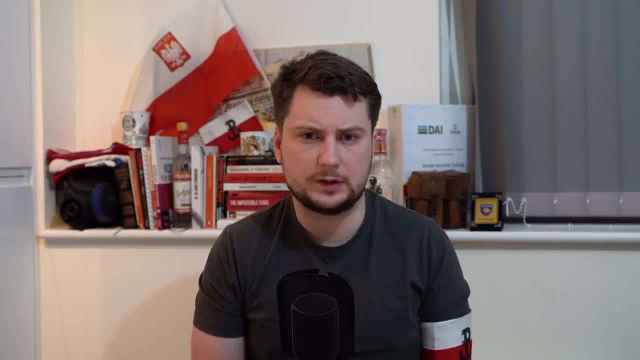 actually as unified as it might seem. obviously, the main thing that actually unites them is the love of polish independence. but, for example, i mean you could see both political parties being there. i saw people from lauren justice and then those from confederation. these two political parties don't like each other and 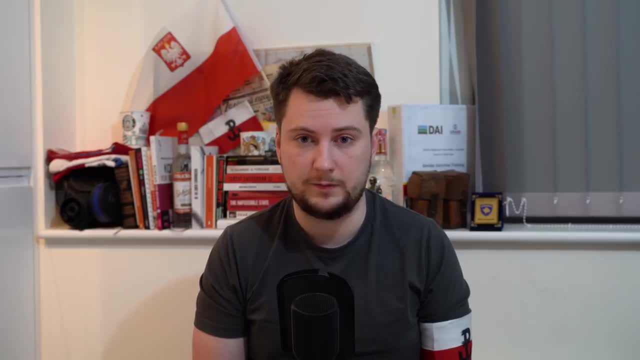 all of various groups. obviously there's even more disagreements. that could go on forever, but regardless it was quite nice to see how a patriotic movement looks, especially considering how rare it is in the uk. but after all that, i did my first ever meetup. lovely to meet you all. 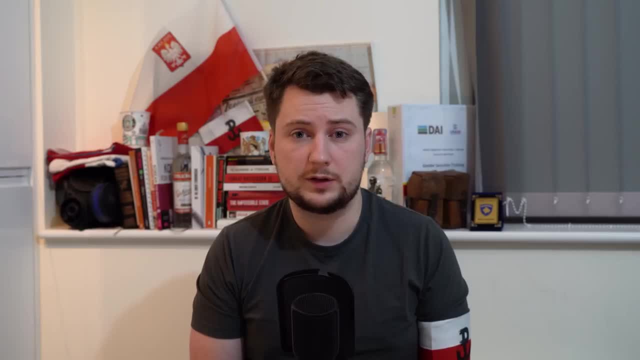 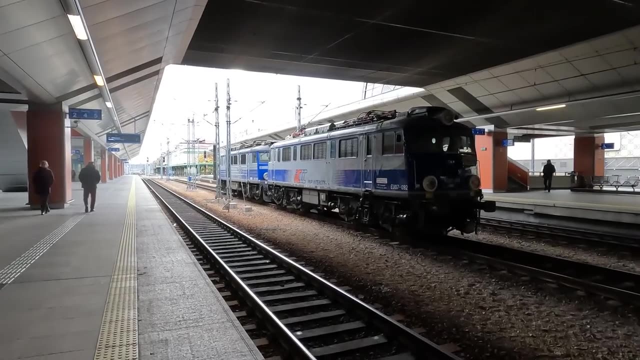 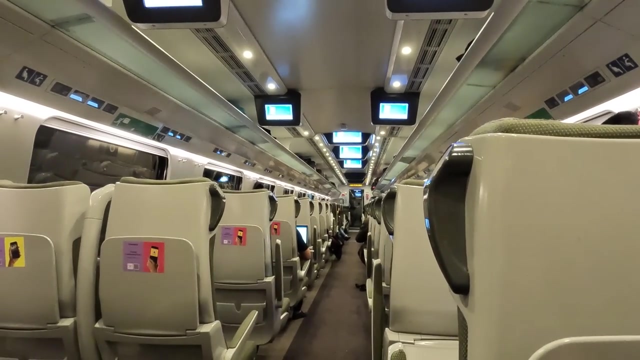 and then it was time to go and see the site most known for dark tourism in poland: auschwitz concentration and death camp. so what you're looking for is on the website, or your website, you have a lot of options for the student visit, which is very fun. how do you go to a student visit? you have a lot of. 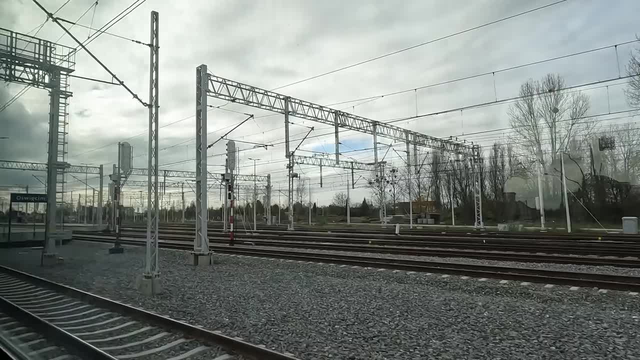 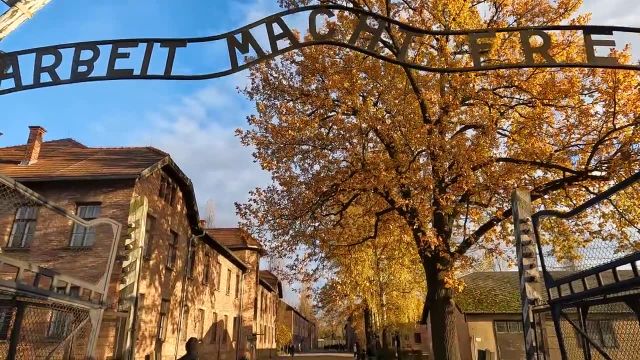 options for students who are doing a lot of work, but one of the reasons why i think it's going to be very fun is that you can get to really enjoy it outside but also really feel at home being in the same place, which is how the student visit sees it. you can get good. 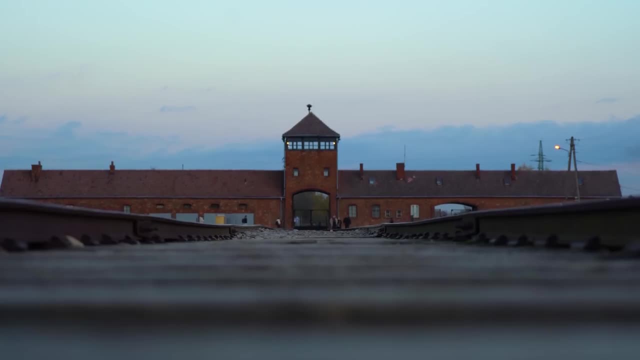 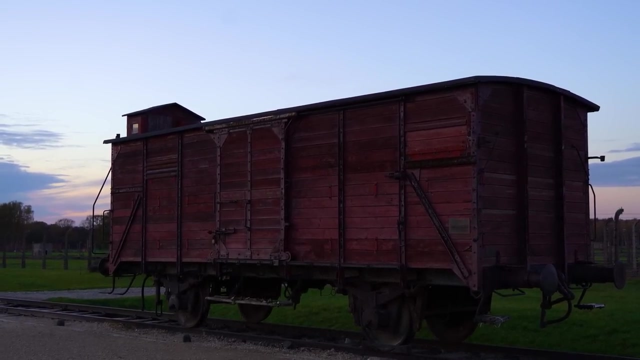 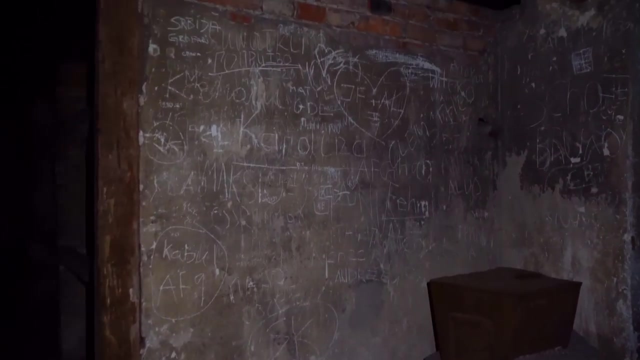 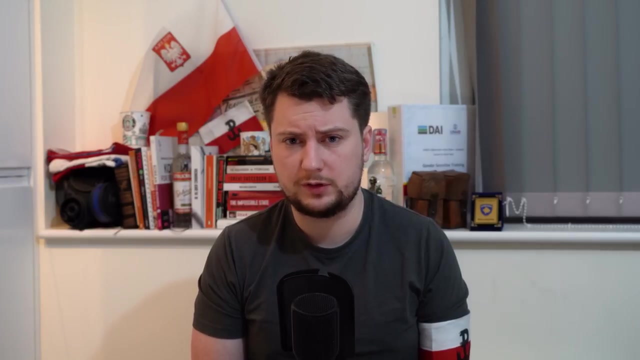 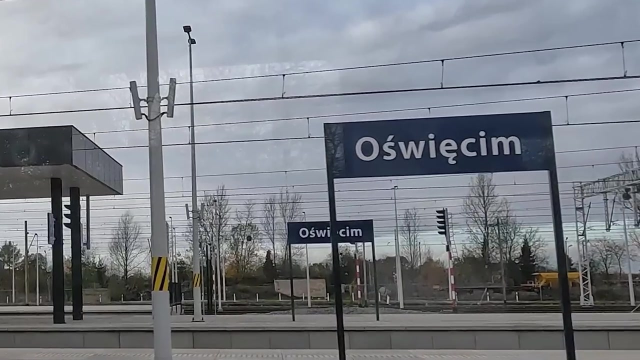 perspectives on what's happening outside. if you can't have a meeting, what could you do? except this place is not called auschwitz? that's a german name given by germans when they tried to colonize the area during the second world war. the polish name i can't pronounce. 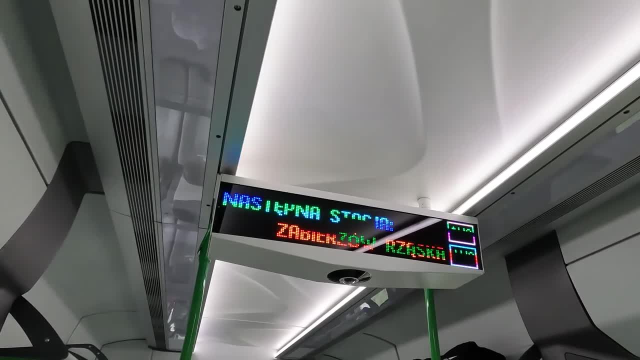 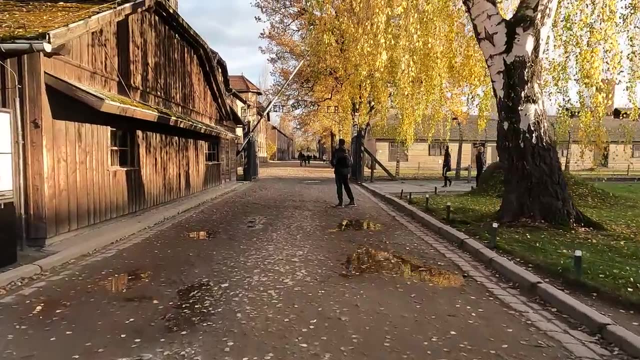 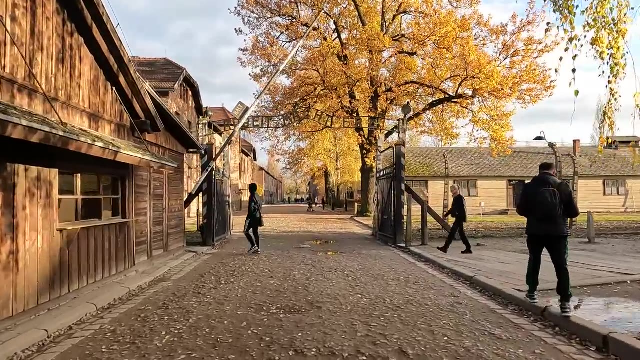 because it's polish, so i'll just let the train announcer do that. when the germans came here, they depopulated the town and set up a 10 kilometer zone in which only they would operate with the ss and set up the first concentration camp, auschwitz one. when the 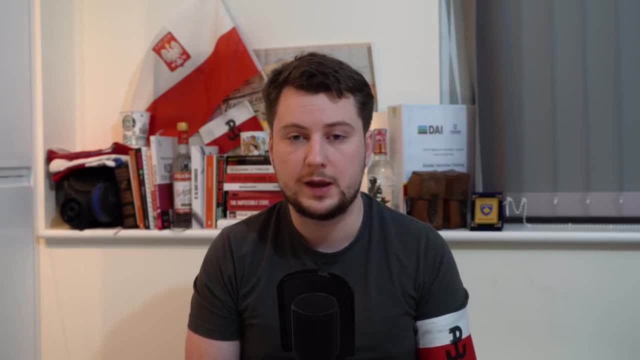 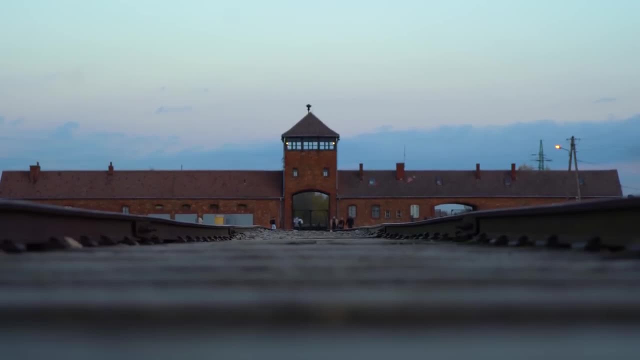 order came for the extermination of the jews and undesirables. this is when auschwitz birkenau was built, which is an extermination camp, otherwise known as auschwitz two. these days, this place does seem to be just your average polish town, but the locals are well aware. 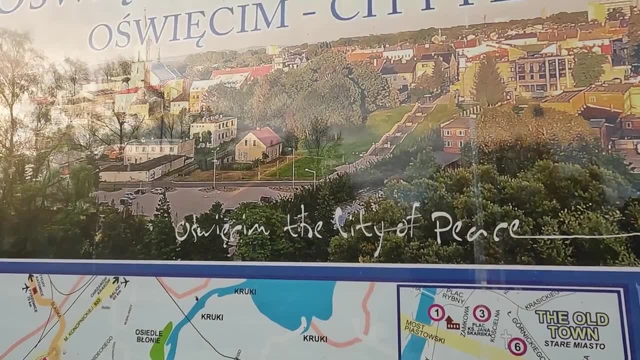 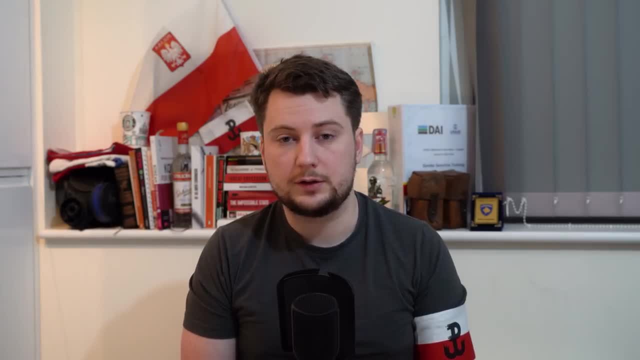 that their only source of tourism is the concentration and death camp immediately after the war. a small percentage of those responsible were put on trial at nuremberg and we still have the camp commandant's transcript from the nuremberg trials. according to the camp commandant, in six weeks, bursts of three trains with 2 000 prisoners on each would turn up daily on the circumstances. those fit to work would fill the empty space in the two camps and those unfits or unnecessary were exterminated. towards the end of the war, the bombing runs knocked out. 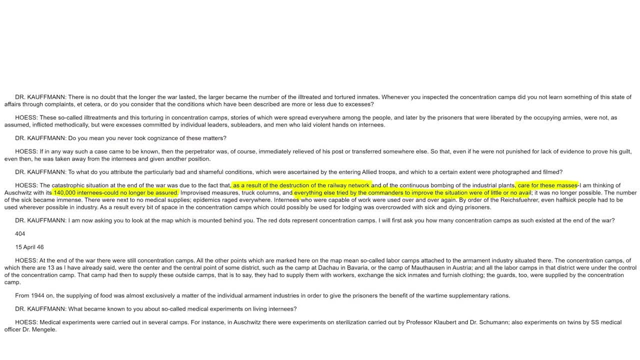 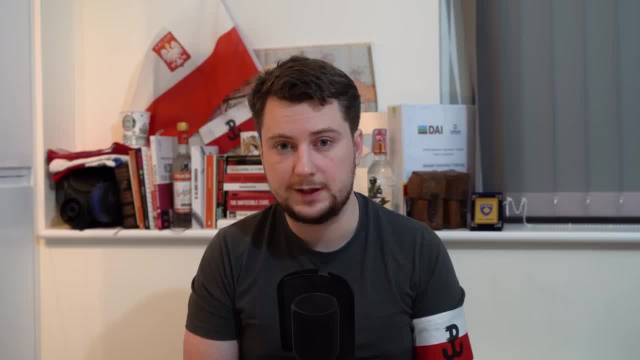 the rail system and logistically it became impossible to continue. after nuremberg he was sentenced to death and the camp was turned into a museum in 1947.. immediately the museum became a political tool. for example, the countries whose citizens were exterminated here were allowed. 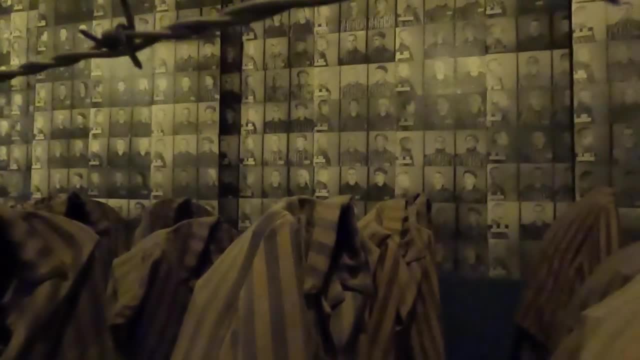 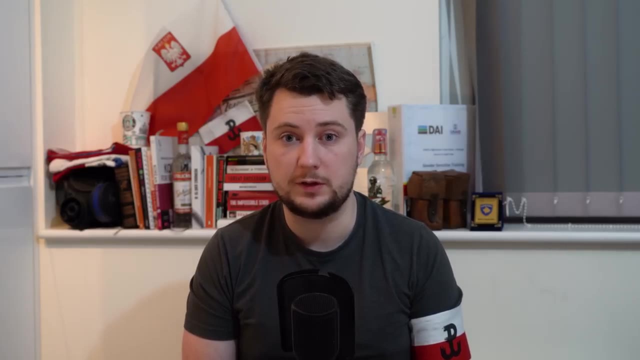 up their own exhibits telling their own unique story and naturally communist countries like the soviet union or yugoslavia decided their exhibits would just focus on victims of fascism. there are claims online as to some of these exhibits, such as there is a claim in the early 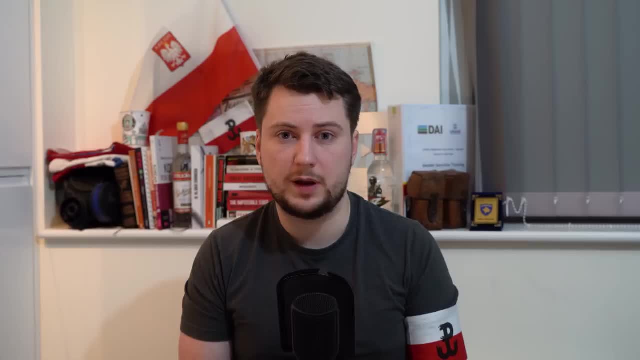 days that the soviet union put on an exhibit to try and compare the conditions of the camp to the conditions of people living in the west. i wasn't able to find a source for that one, but for definite. the whole situation became incredibly politically complicated, especially. 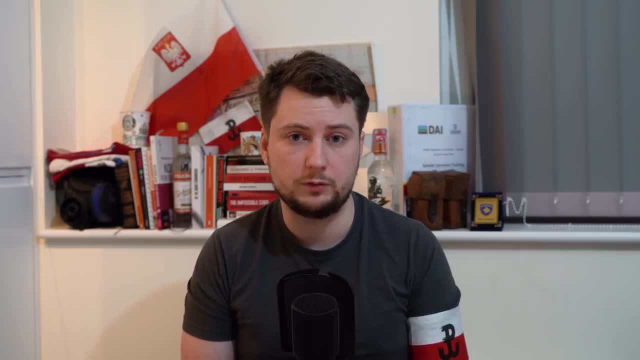 after the soviet union and yugoslavia collapsed, as to who would be allowed to set up exhibits and what would be allowed to be shown. for example, with the yugoslav nations it was agreed upon that the former yugoslav nations would have to agree on what the yugoslav exhibit would be. 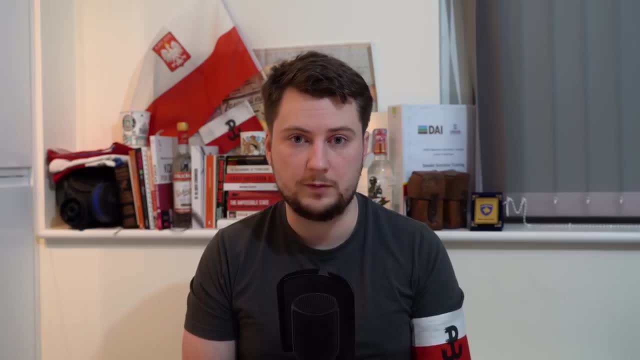 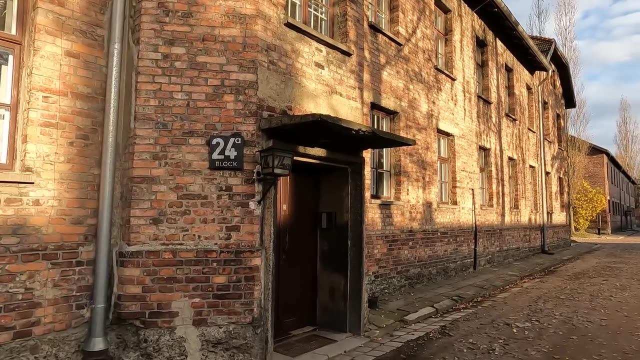 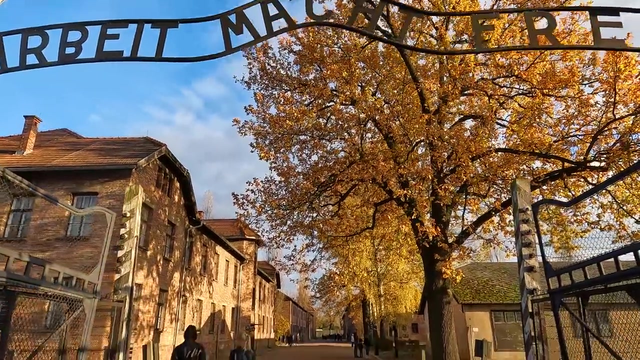 naturally, they couldn't agree on anything and nothing has been shown since visiting. you will be met with the concrete building that is the visitor center, before you walk down to the surrounding buildings used by the camp and its guards, and finally, the entrance with the work sets you free, in metal letters above you as you travel from building to building. 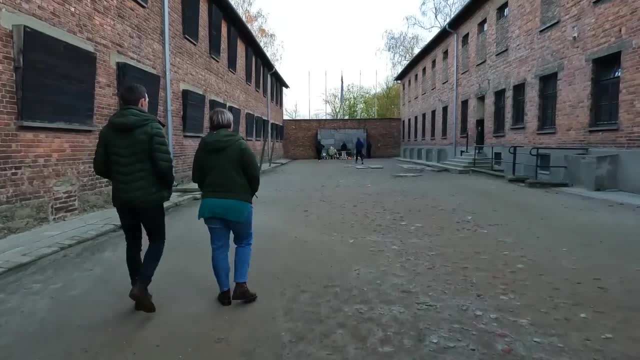 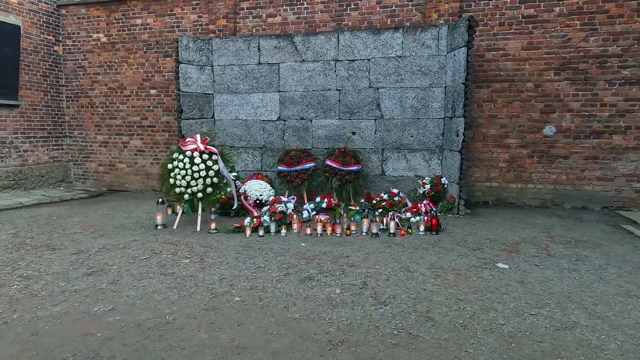 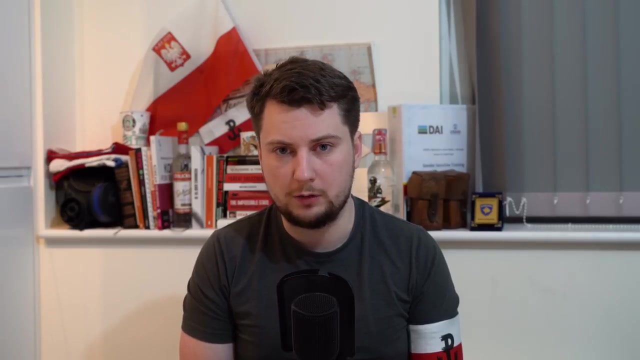 you can learn about the specific horrors that took place, such as the execution area known as the death wall. about 15 000 polish citizens were shot here, and about a thousand soviet citizens. many of those were polish resistance fighters, with the most famous last words being: long live poland. 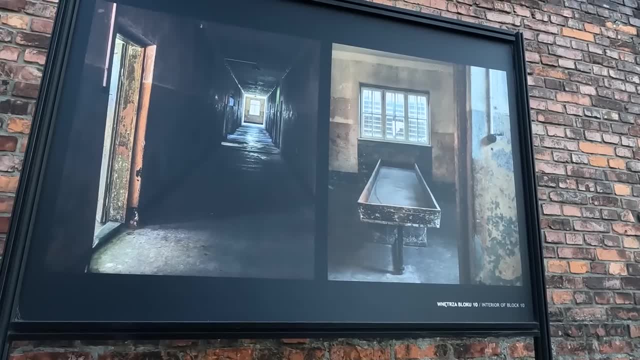 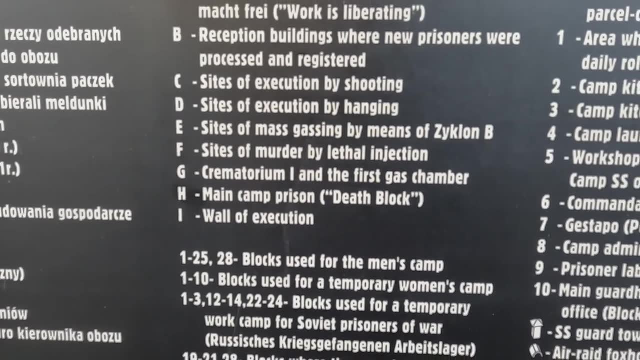 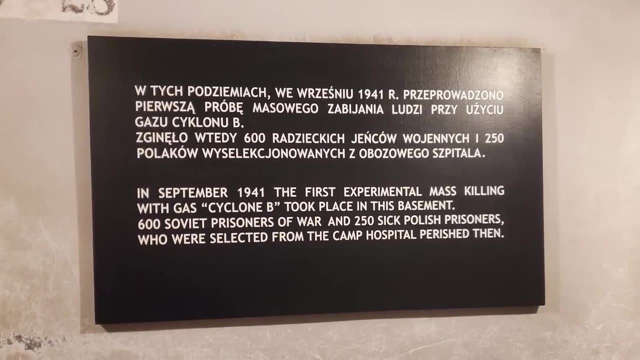 there is block 10 for medical experiments- a lot of dead kids- and then block 11 for the punishment block, a place of not only immense suffering but the birthplace of the use of zyklon b, as it is listed as the location in which it was first tested to exterminate prisoners. but 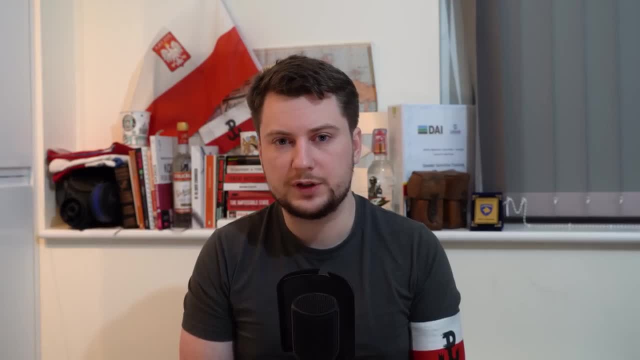 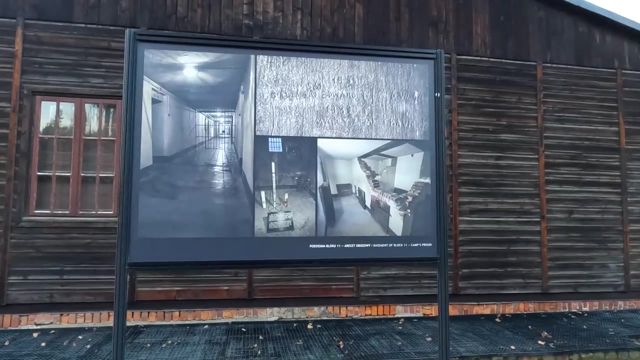 it is also a place of immense heroism. when a prisoner escaped, 10 would be selected for death. and so, as a polish sergeant was selected for death, he began crying about his wife and children, and a bishop stepped forward to take his place in the cell where he was murdered. a monument to his heroism still stands. it was at. 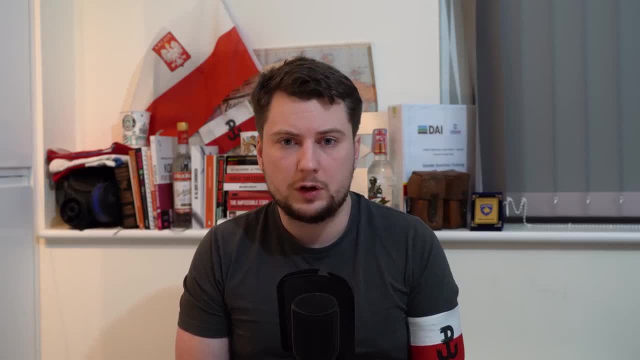 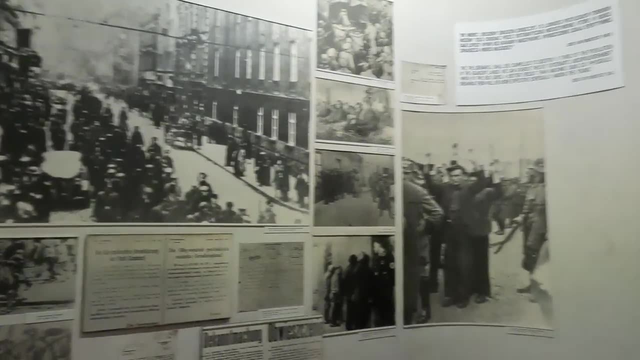 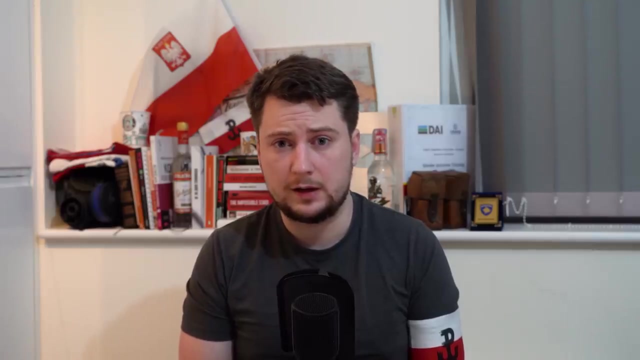 this point that i began to notice that these polish stories are something i'd never heard before, and in fact one of the buildings was converted into an exhibit entirely dedicated to polish resistance during the war, and even in the camps, polish resistance was truly legendary and ran by some serious mad lads. one of them even decided to volunteer. 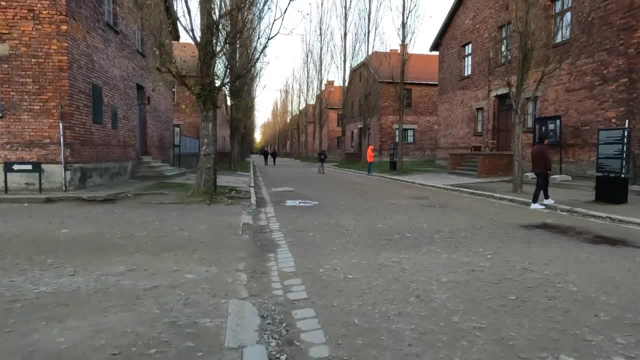 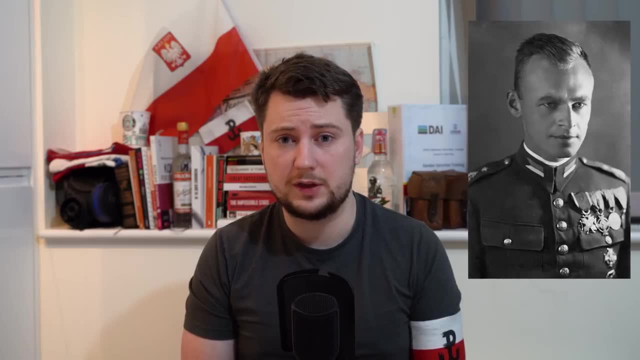 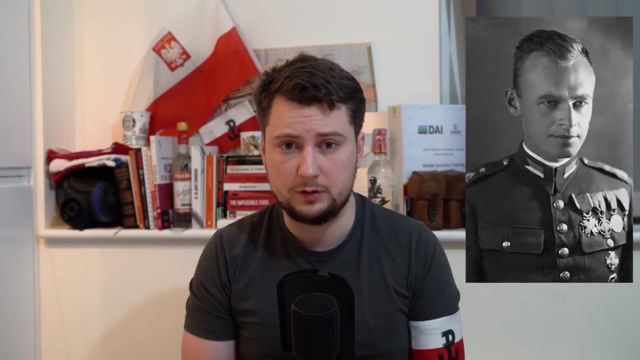 for a mission in which he broke into auschwitz with the dedicated goal of setting up a resistance movement within the camp. sadly he failed and had to leave. but this guy then went on to fight in the warsaw uprising and even continued his resistance against the soviets until his death- absolute mad. 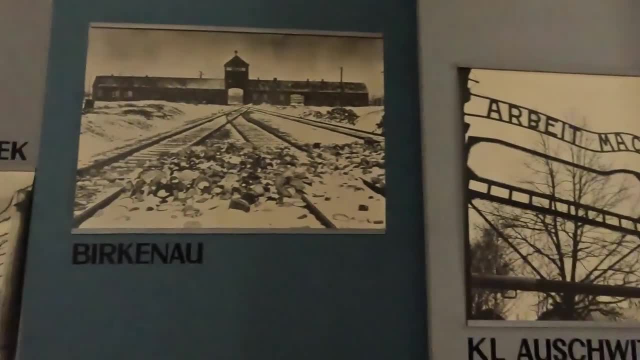 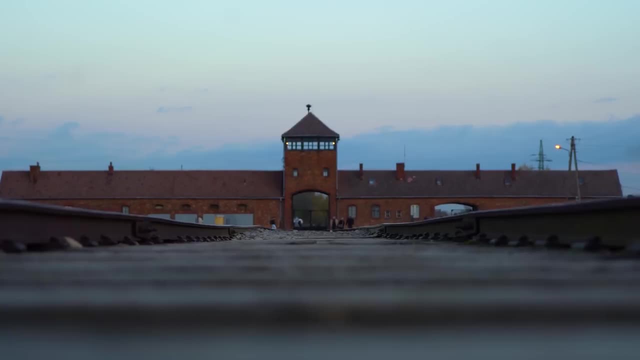 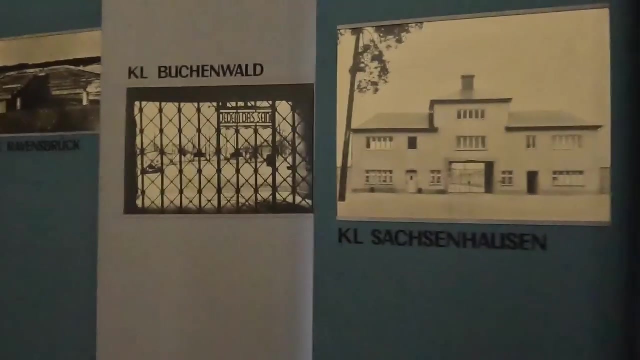 lad. camp one, however, is nothing compared to auschwitz-birkenau camp number two. camp two was a purpose-built death camp, and it is the reason auschwitz is the one death camp everyone can mention. The National Socialists set up hundreds of different kinds of camps for different 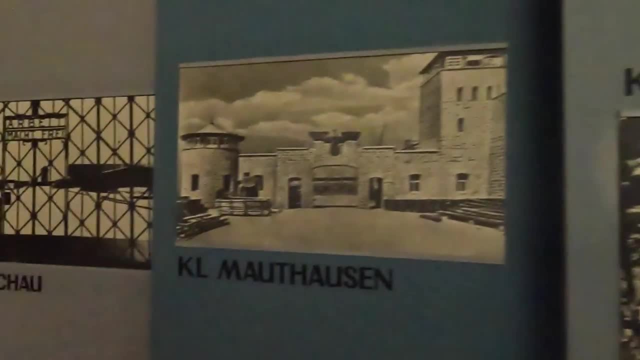 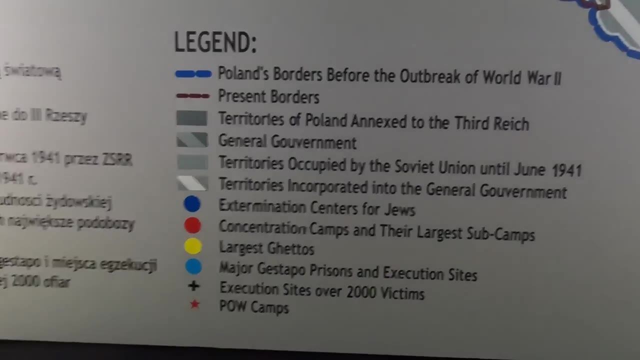 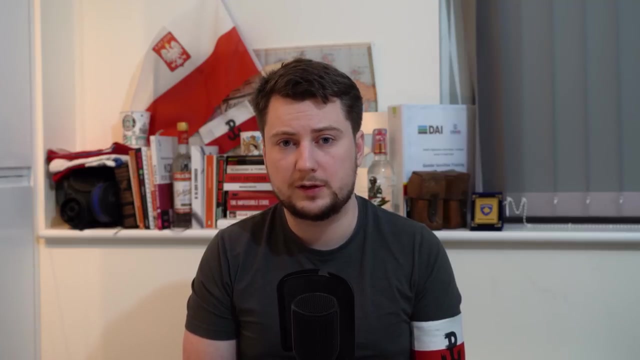 purposes, but only six were extermination camps. Auschwitz Camp 2 is the one that killed the most people, making up 35% of all extermination camp deaths, at an estimated 1.1 million, around 90% being Jews. For perspective, this is about 400,000 people less than those who died. 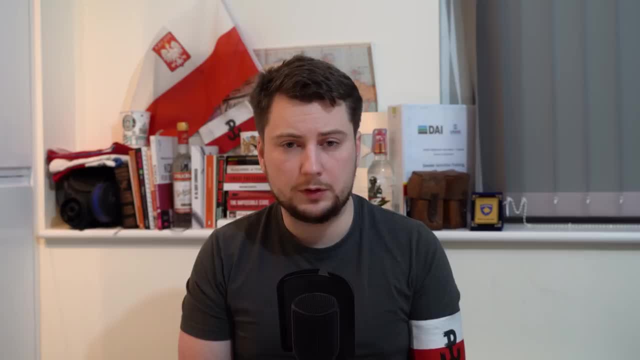 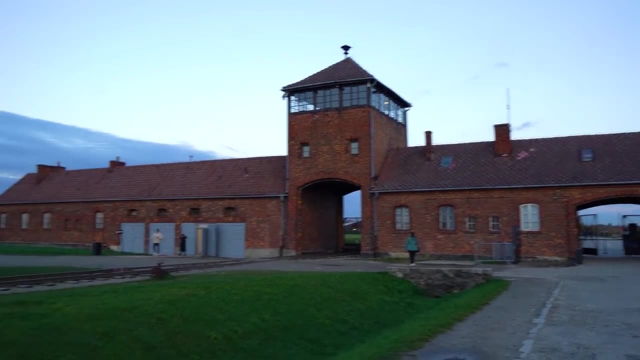 in the Battle of Leningrad World War 2 was not fun. To get there you have to take the Auschwitz bus and once you arrive and walk through the famous entrance, the sheer scale of the thing hits you. The very centre is an area for train drop off. 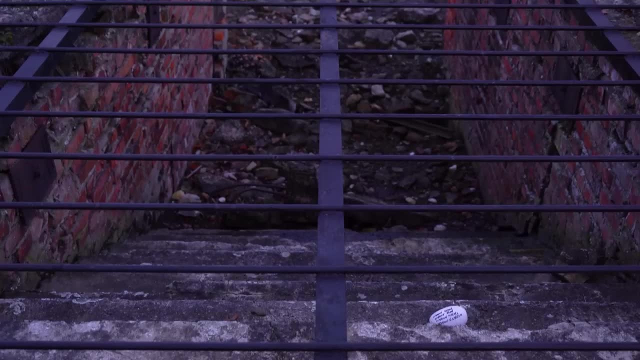 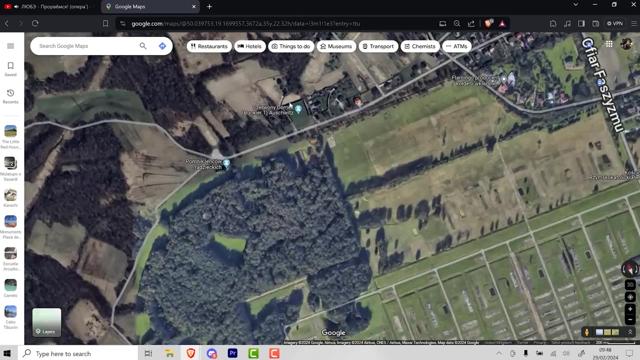 there is a single wagon left in place in memory. Walking through the camp, I eventually came to a gas chamber. Initially, the exterminations were done in the Little Red House, which was a converted old house nearby, but then four professional purpose built gas chambers were built inside. 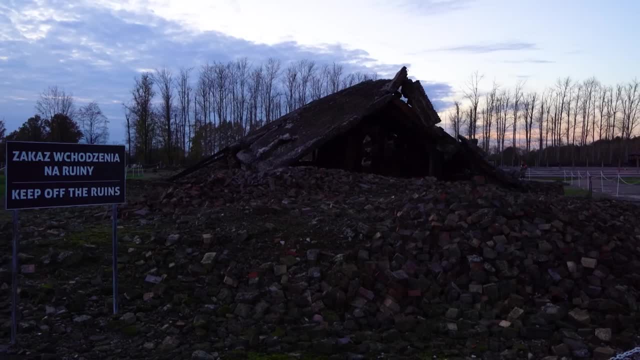 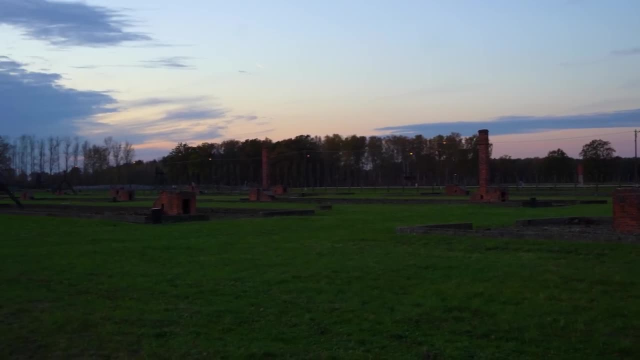 of the camp grounds and then the exterminations were done in the Litter Red House, which was a much closer to the drop off point. Now they are largely rubble. In fact most of the camp is rubble, and what is left is even smaller than what happened at peak size of the camp. and you can see. 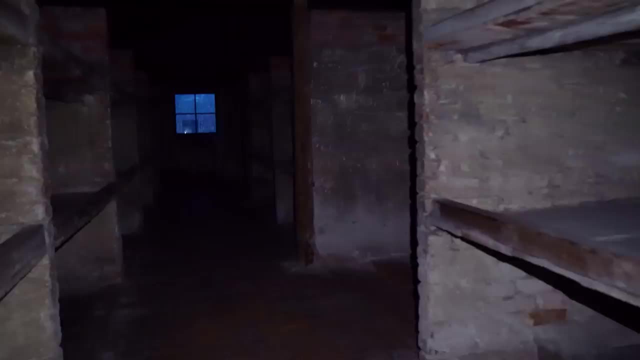 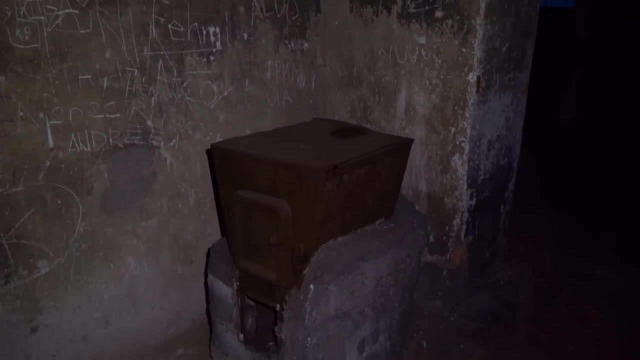 this in aerial photographs of some of the downsizing, But it was approaching closing time and the last thing I wanted to do was check out some of the buildings where prisoners were kept for work detail And, given it was winter, it was already getting incredibly dark And I have to say 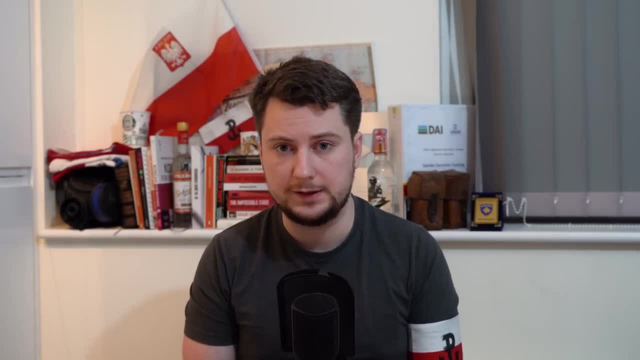 an extermination camp in the dark is probably the worst thing you can do in the world. But with that it was time to go and thanks to time constraints, I wasn't actually able to see everything I wanted to, so I certainly recommend leaving a full day to actually experience both. 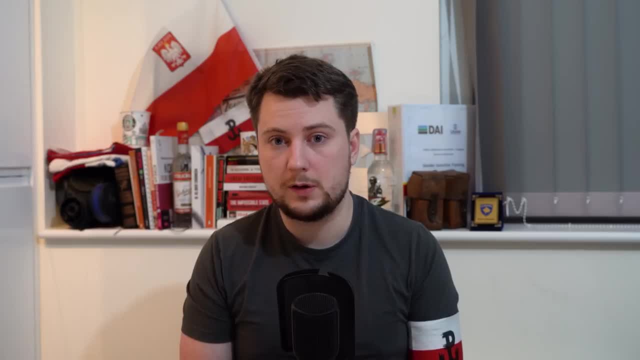 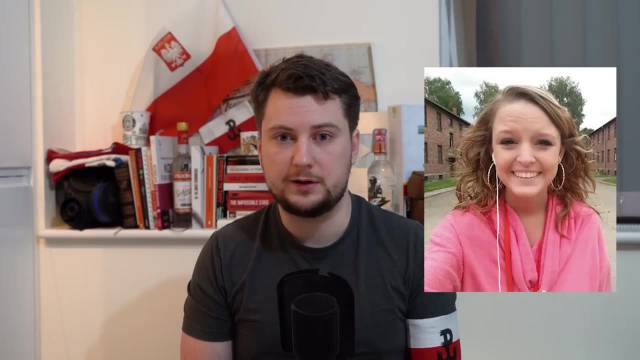 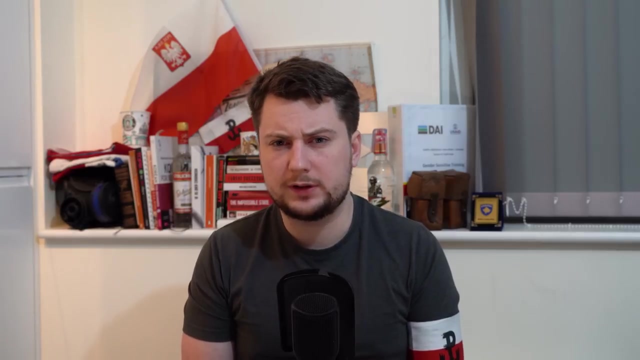 camps in their fullest. But if you are going to go, what of advice? Remember it is an extermination camp. Don't take smiley selfies outside of it. Apparently, this is a routine problem, especially with women. They really, really don't like that. This trip, however, did leave me with a bit of a 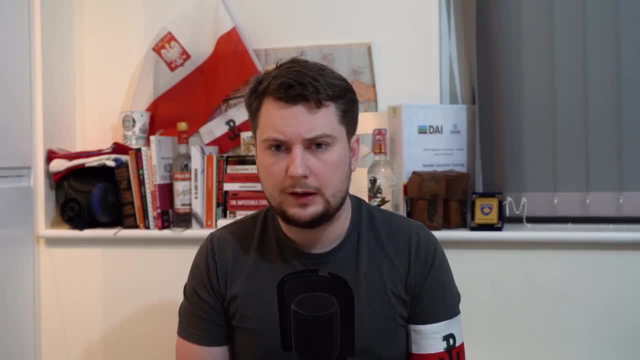 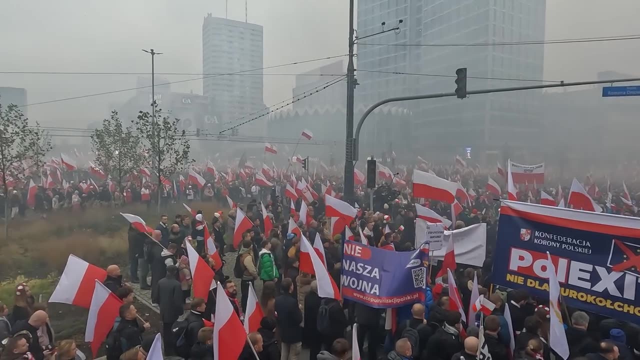 few opinions which um bugger it. this video is not getting monetised anyway, is it? Polish Independence Day was truly something to behold and something that you have to feel quite proud for the Poles for having, especially with everything they've been through, It's sort of their 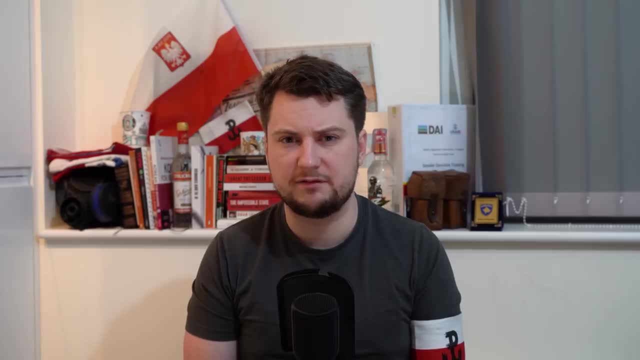 way of saying that we're still here despite everyone and everything which I should have to respect and, frankly, I just hope they can keep it. As for Auschwitz, I can finally understand what people mean when they say you have to see it in person, for example. I think it's a bit of a. 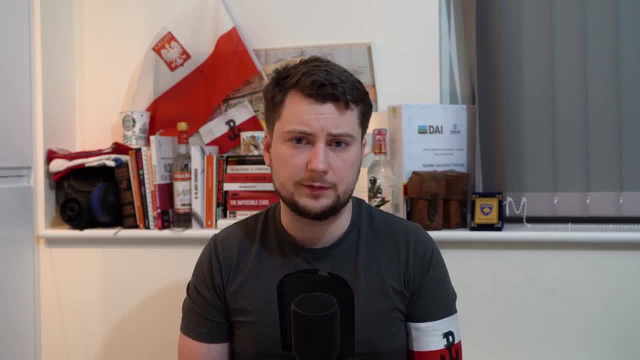 shame that you can't see it in real life. and this isn't like most things where it's just the difference of seeing it on TV versus in reality. I really think that most media and films have a difficulty in conveying the reality of this place to the audience, and I would put this down to the 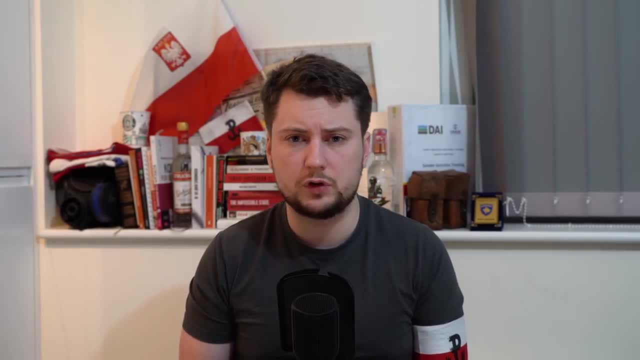 fact that most of this is done through two perspectives: either the Jewish perspective or what I'm going to call the German perspective. The German perspective is one that is incredibly dry, in which the pure facts and figures are told, the story relayed and leaves you with a feeling of not really understanding how this happened. 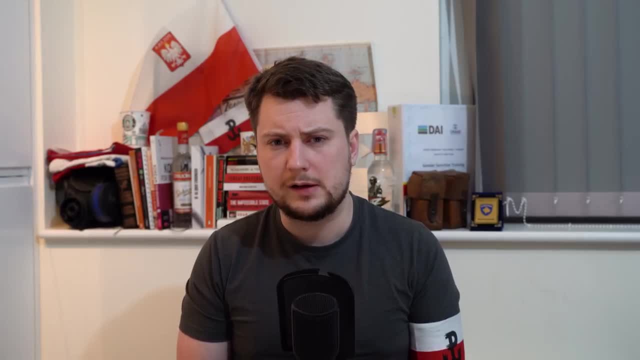 and also a feeling that it is not to be discussed again, which doesn't convey reality. What I would call the Jewish perspective is something that leaves you distraught as to how something inhuman could actually happen and leaves you with an almost physical sickness that means that you're 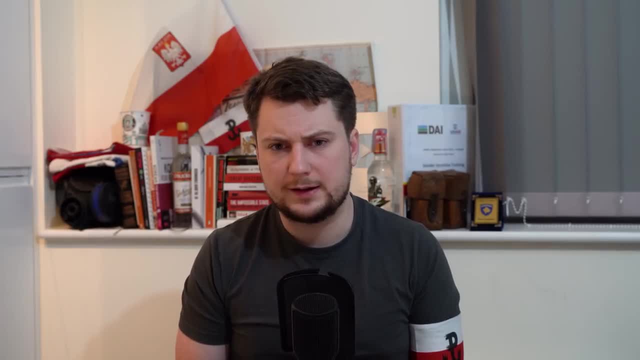 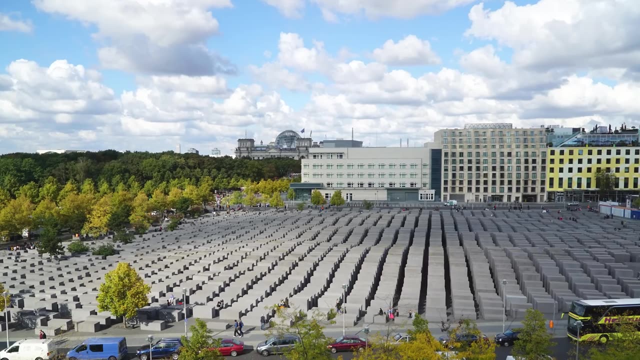 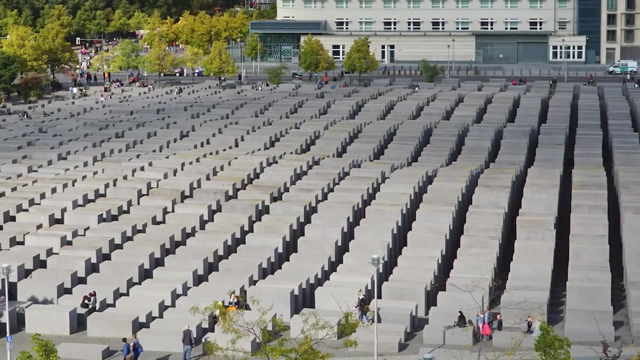 not really able to comprehend how this could have happened, And I think this feeling can be most easily described through Holocaust memorials such as the one in Berlin, which is made up of these unnerving concrete blocks with walkways between them that leave you utterly disorientated and 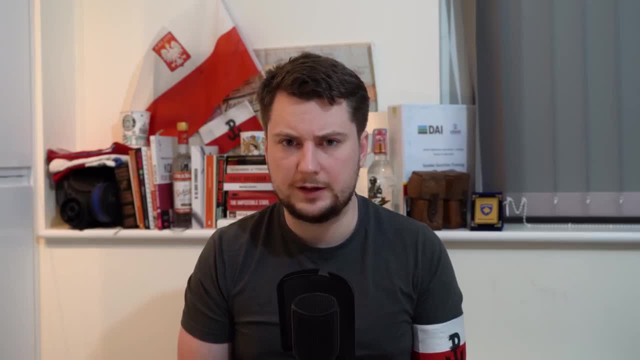 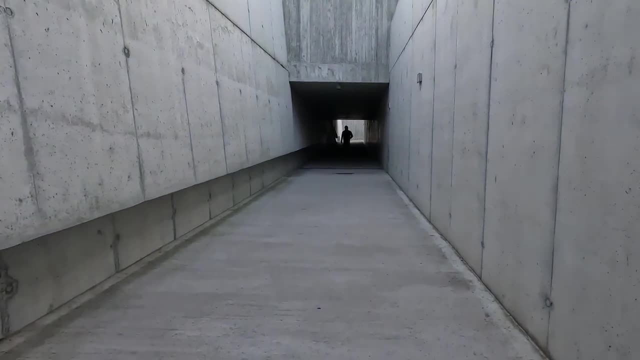 distraught by the feeling of even being there, And you can get a similar feeling when you visit the Auschwitz Museum. The entrance is made up of a long, featureless concrete hallway, with the only thing that you can hear is the names of the various victims. 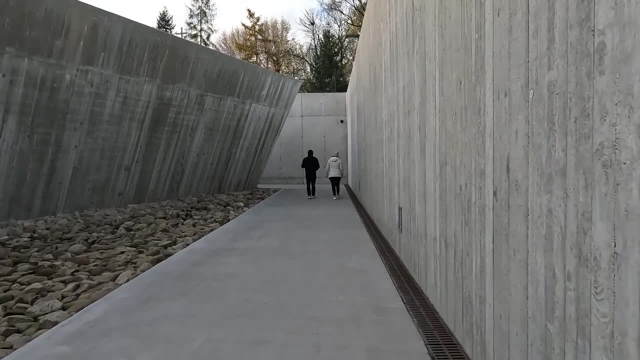 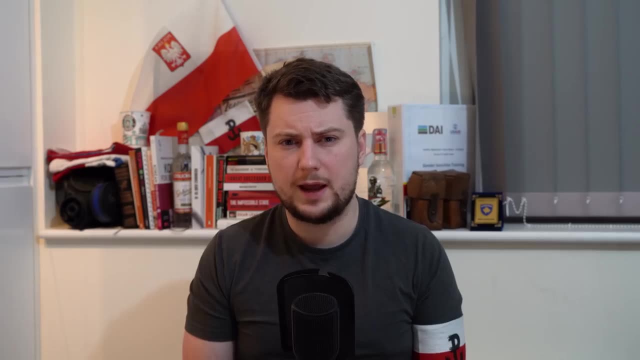 Moszek Kwar, Antoni Folon, Pavel Flitman. Whereas when you're in the camps, they're not featureless, nor are they incomprehensible. Instead, they're a very real place in which you can get a sense of what happened here. 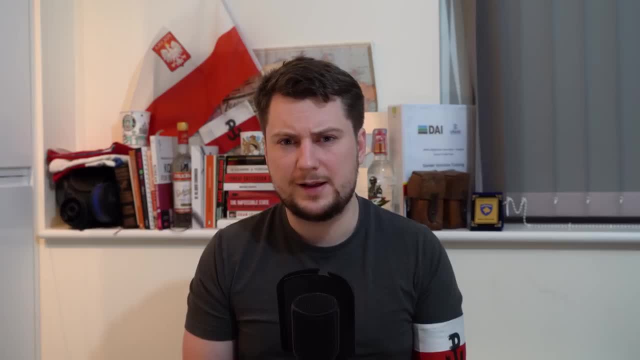 and how and why it happened, And in which case that feeling is something unique. In fact, I've only ever felt it once before, when I watched a movie called Conspiracy about the Wannsee Conference. The Wannsee Conference is where a group of Nazis met to decide on how they would exterminate. 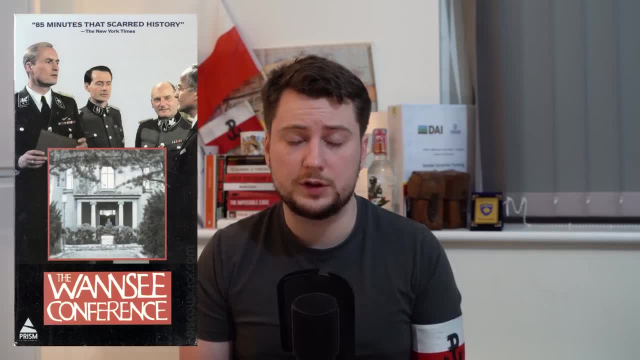 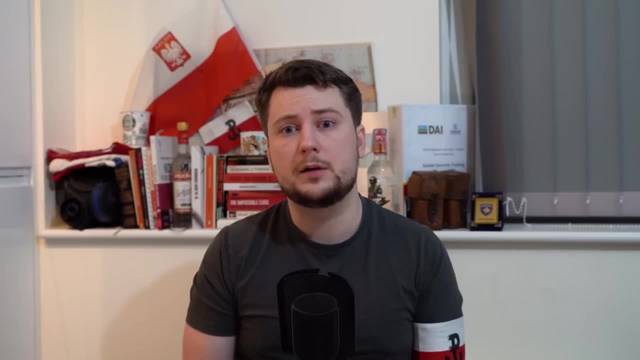 the Jews. There is a German version of the film which is incredibly dry and poorly reviewed because it feels like you're watching some kind of courtroom reenacting of what happened, whereas the British version actually allows the people playing those roles to have characters.